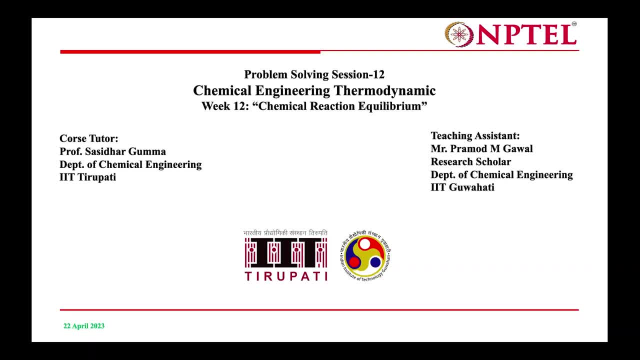 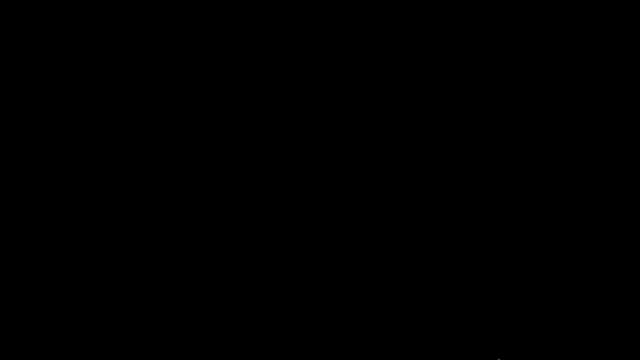 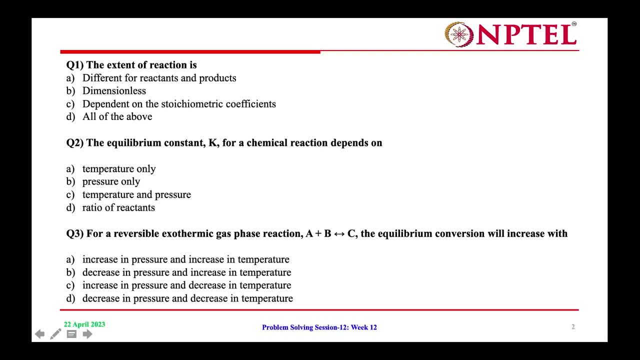 one To ask the question one: the estado reaction, each of scenario, the different reactant and products that miss knowledge dependent on the stoichiometric coefficient, on theало, Basically, stop reaction. reaction is the same For the all the elements. this is not a, it is a. 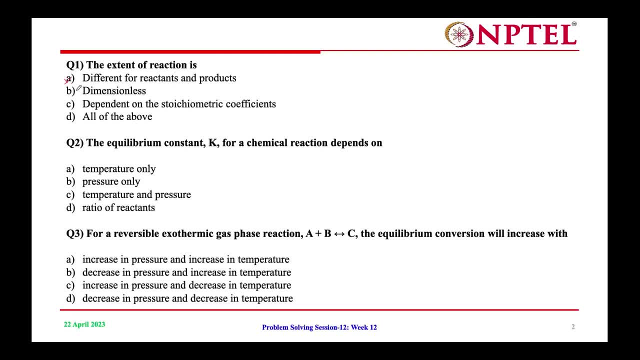 uh, the unit of the extent of reaction moles, and c is a dependent on the stoichiometric coefficient. this is the right ones. so is equal to d? n? i over v? i. this is a stoichiometric coefficient. n? i? n final means moles of final moles divided by 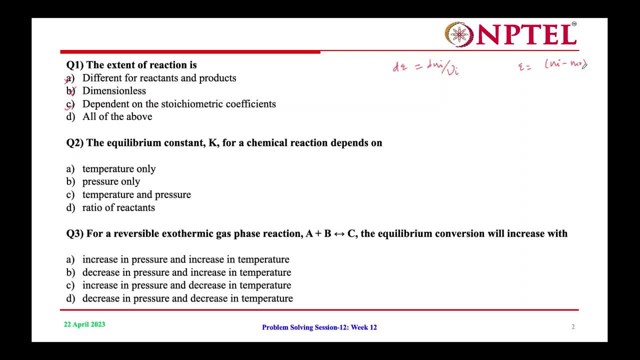 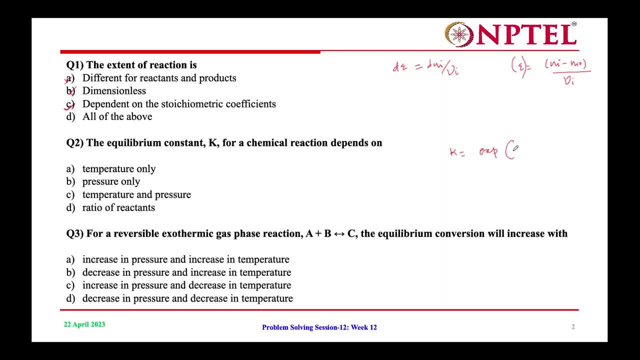 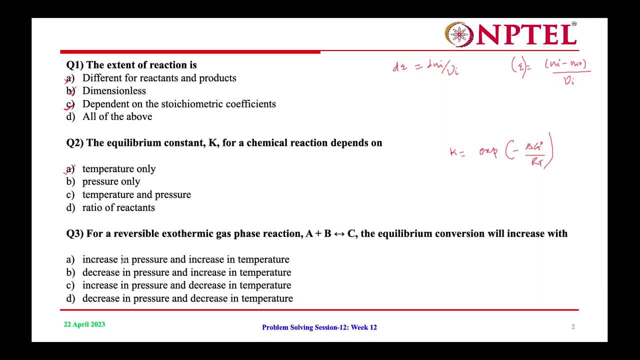 you see, the equilibrium, uh equilibrium conversion will increase with option are given. will increase with option are given. will increase with option are given. increasing in increase a pressures, increasing in increase a pressures, increasing in increase a pressures and increase in temperature and increase in temperature and increase in temperature can be decreased in pressure and increase. 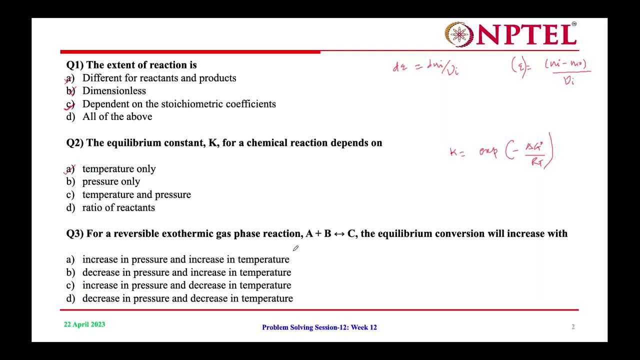 can be decreased in pressure and increase can be decreased in pressure and increase temperature. so, before going to the option, we say so. before going to the option, we say so. before going to the option, we say: product submission up equal to equal to equal to stoichiometry coefficient. 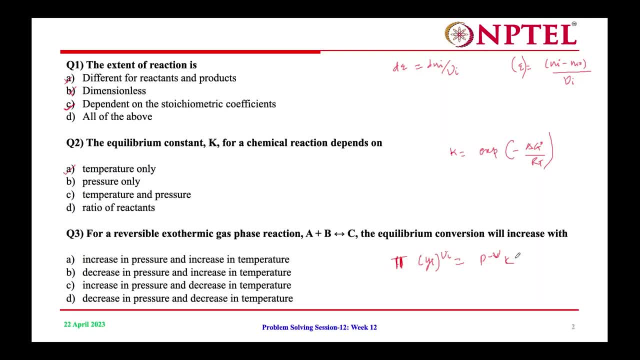 stoichiometry coefficient. This is the product notation. like, for example, pulse 5 is equal to 1 to 5, here is the add 1 into 2, into 3, into 4, significance of this time. this is the product notation, so exothermic. 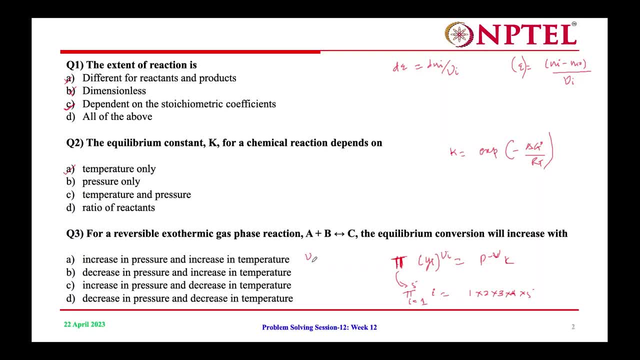 so here total psychometric coefficient equal to minus 1,. here is the reactant. here is the reactant of a minus 1. for b plus c it is a minus. so here total psychometric coefficient is negative. so it gets positive. so it gets positive. 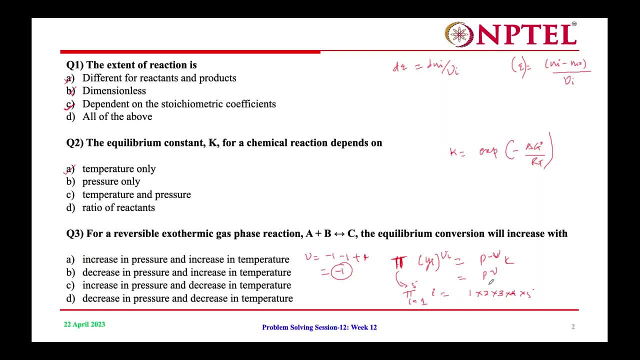 So it means that pressure is increased, right, and decrease in temperatures because here so here. so it means temperature decrease, right, So here equilibrium conversion will increase. the option is c means the equilibrium conversion will increase with in the increase in pressure and decrease in temperature for the exothermic. 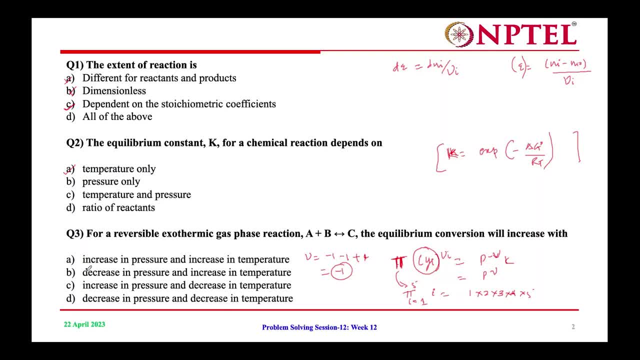 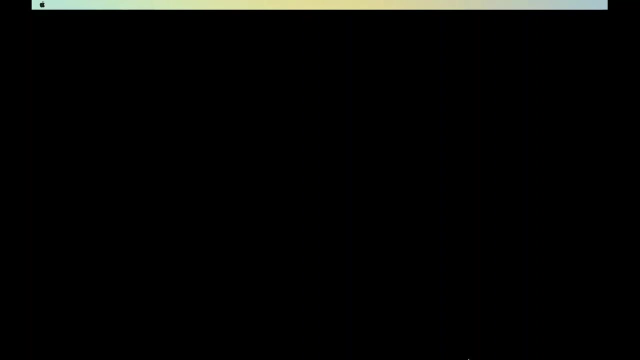 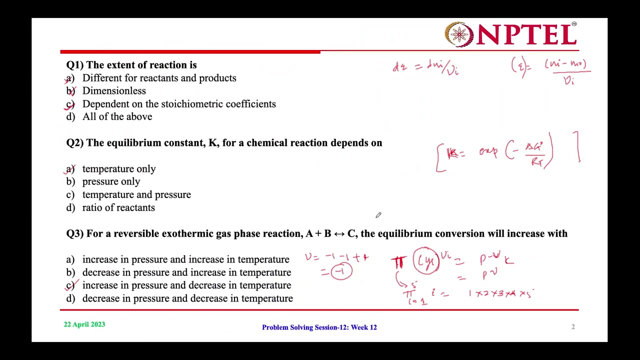 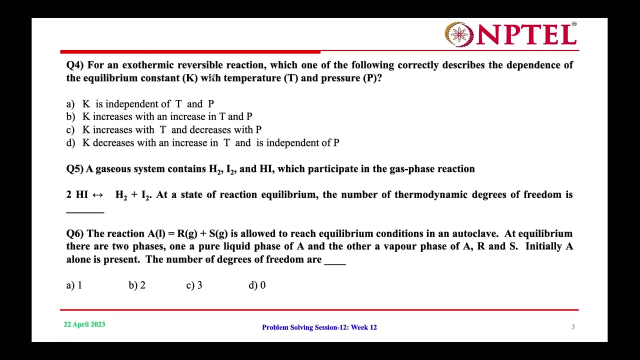 reaction. right, I hope you got this Now question. coming to the question number 4, for exothermic reversible reaction, which one of the following correctly describe the dependence of the equilibrium constant k, with the temperature and pressures option are given: k is independent of t and p. k increase. 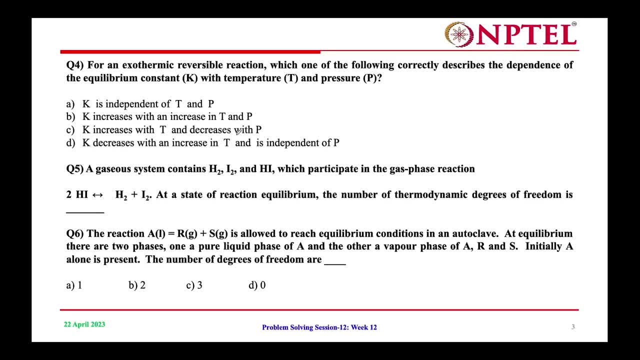 with increase. t and p k increase with t and decrease with p and d d k decrease with increase. We know the relation: k by k1, delta h r, 1 by t, 1 by k1, right, so we know the relation. 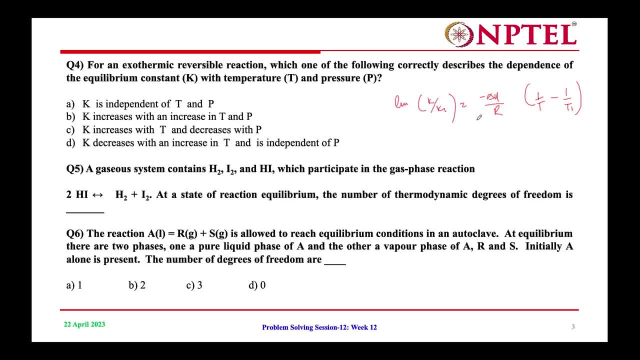 k by k1, delta h r: 1 by k1, right. so for exothermic reaction delta h is a negative, hence with increasing temperature k decrease. for exothermic reaction And for endothermic reaction delta h is a positive, so k is increase with increasing. 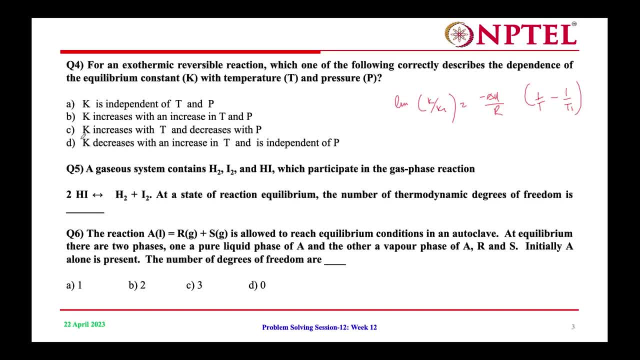 temperatures. So for the exothermic case, decrease with increase temperatures and in and it is independent of the pressures. I will have to clear If anybody did get. anybody didn't get clear with us. question for you. a gaseous system contains is to i2 and h i which participate in the gas phase reaction twice h. i use h. 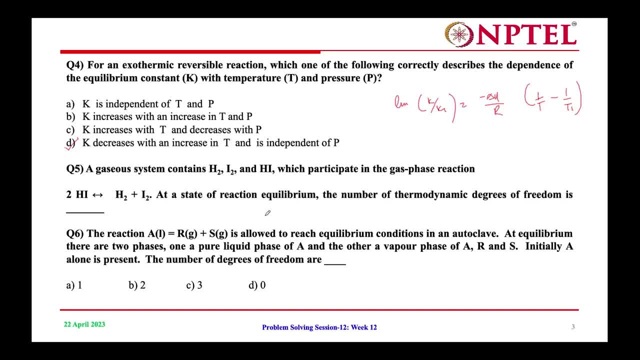 2 plus i 2, this is the irreversible reaction at a state of reaction equilibrium, the number of thermodynamic degree of freedoms. So here a given a number of component: 3 is equal to 3 and phase is 1. right now, here is. 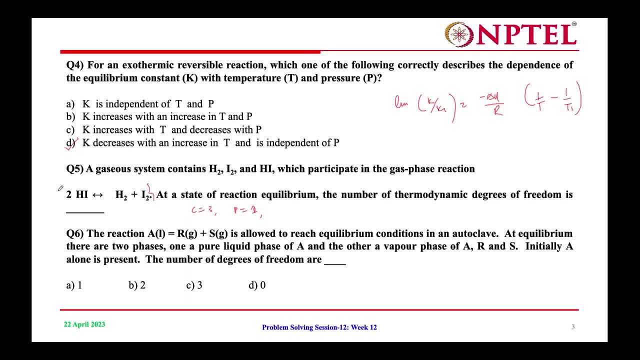 a 1 independent reactions. so that denoted by So number of degree of freedom equal to 3 minus p plus 2 minus 1- sorry is a r is a number of independent reactions. to put all the value in this equations: p minus 1 plus 2 minus 1. 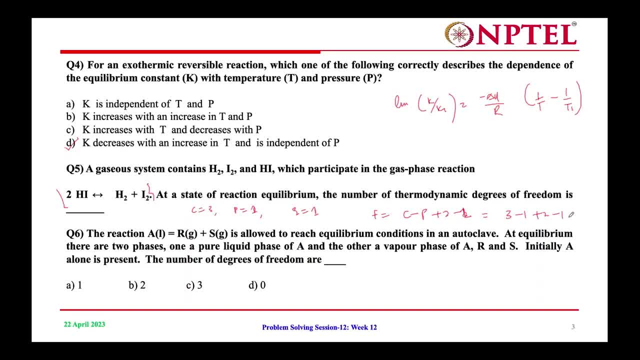 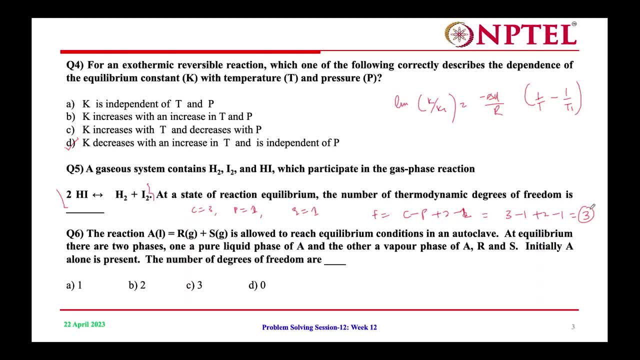 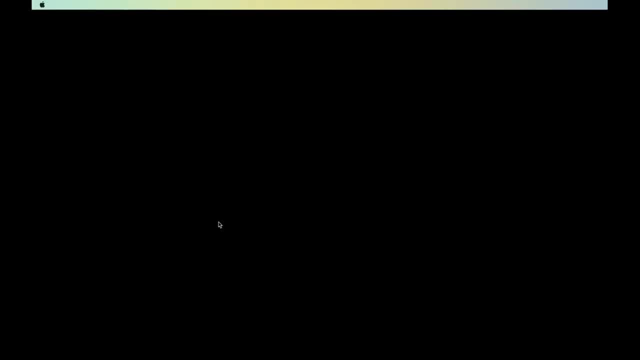 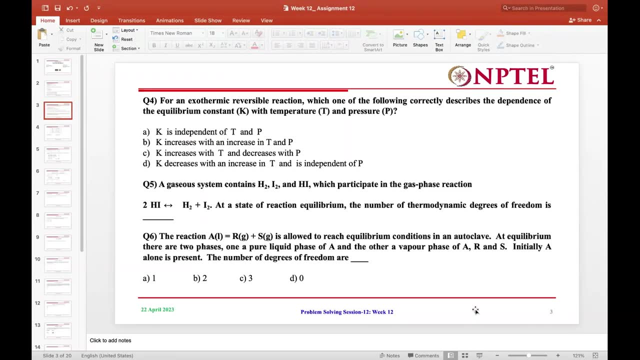 сл Tae짱 case is the frames of this unit. So let us trace up high p versus low p, our capital Ra. Well, did the other part at 처음. from here, at when is this x and this Zeta case? So let's discuss g, maybe the same another factor minus 1 and zeta x. So if I am going to find it in this material is negative value and if I can calculate up to x, zeta, zeta x values in radius, zeta M and Zeta x is negative value. this 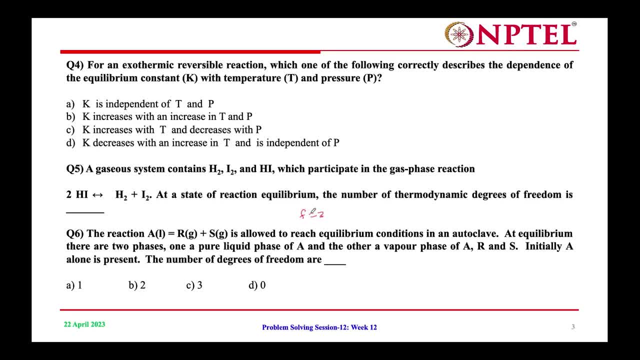 same as X, i2,, f and beta times. c2 of the neutral time initial factor angle is equal to three. that's the temperature, pressure and mole fraction. question number six: it is similar to the question five. the reaction a gives to r plus h is allowed to reach equilibrium. 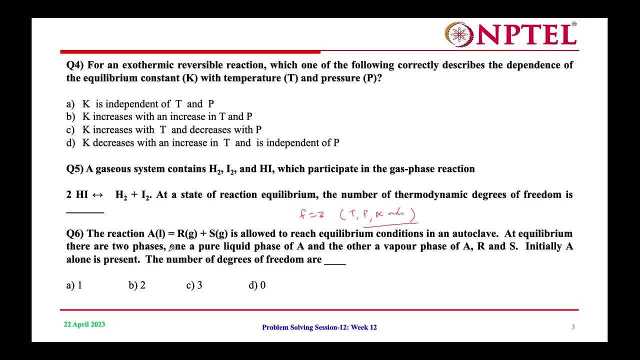 condition in at equilibrium. at equilibrium there are the two phases, two pages, one for liquid, phase of a and other vapor phase, a, r, and yes, initially a alone is present. the number of degree of freedom, r. so here same formula: f is equal to c minus p plus two. 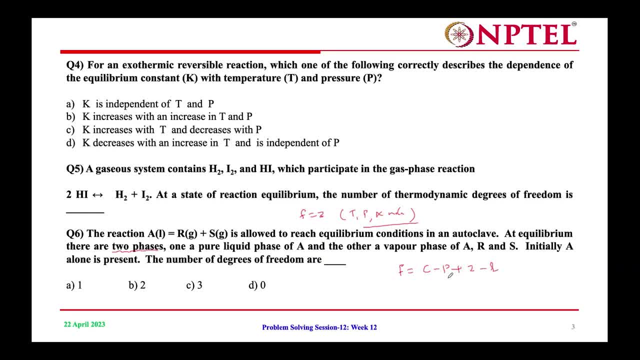 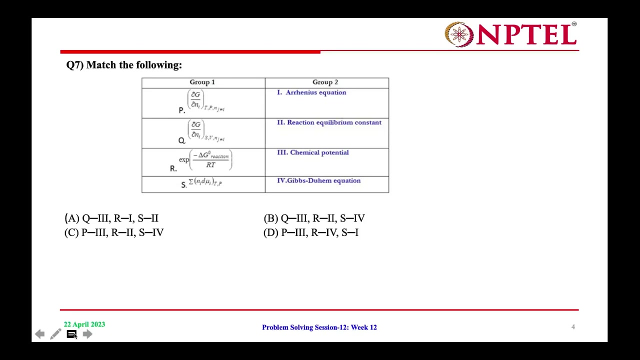 plus r a number of independent. so here is a one here. number of component three and phase is two, a minus two plus two minus one. all of you got clear. am i audible to all or not? coming to the question number seven, match the following here: group one and a group. 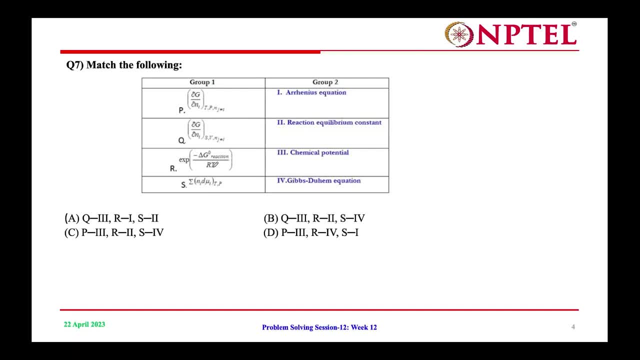 row, but here the given the uh equations. they have to match you. these are all we have to write down, and this is the grandmother struggling with the Mädel, in sequence till the theท: elle: dG divided by di cap and exponential minus delta. g. reaction divided by rt, the reaction equilibrium constants. 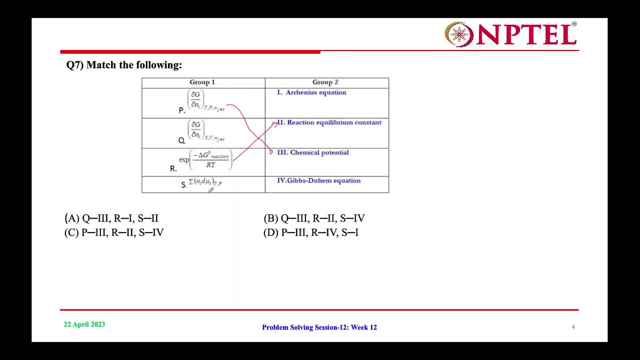 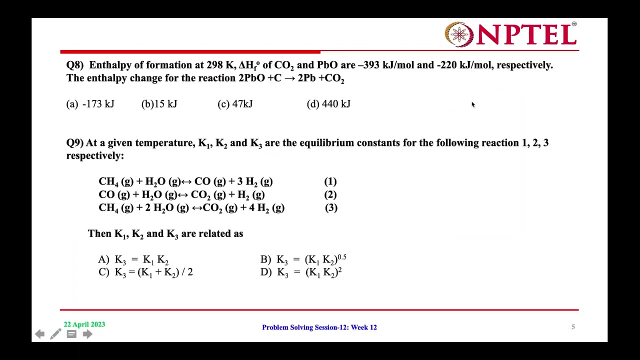 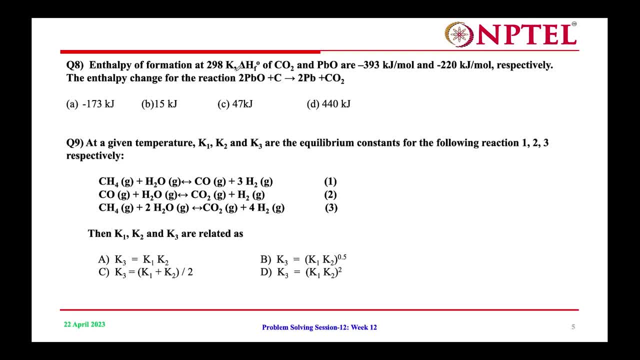 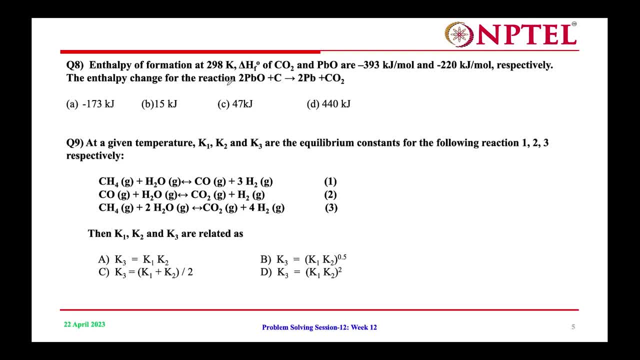 per mole respectively. the enthalpy changes for the reaction twice p. pbo plus c gives 2 pb, co2. so enthalpy of formation given for pb and co2 here. so you have to calculate enthalpy change for the reactions you. you calculate the change of enthalpy for these reactions. delta h. 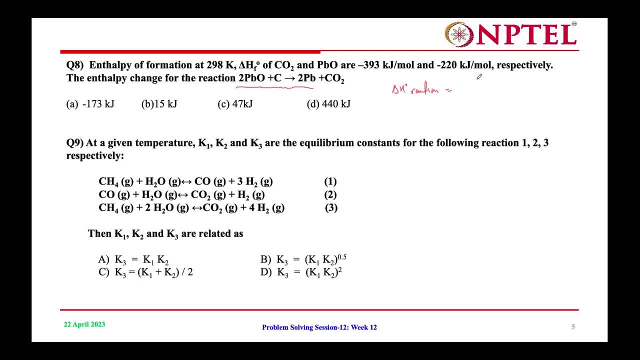 reaction: delta h product minus reactant. it here, they're here for other toy: 2 pb zero plus plus co2 given for pbo twice into minus 220 plus zero, so 27 kilojoule. so 27 kilojoule zero plus one. 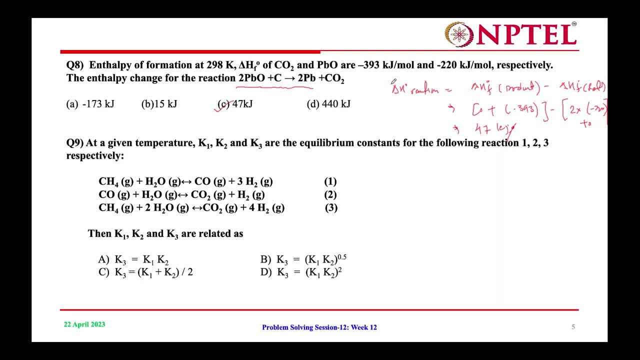 this channel equation you can calculate. so you could calculate it r into alpha without using ain to use seen over l. I'll have to try how to how to solve this one. this is a chemical reaction number one, two and three. suppose we add equation one and two here, so CH4 then CO, CO gate cancels here H2 twice H2O plus CO2 plus 3 plus 1, 4, right? 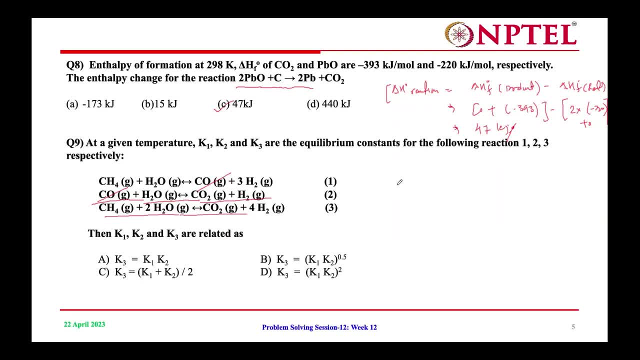 this is valence equation. so when, when we add the one and two gives the equation number three right. so delta g 3 to delta g 1 plus delta g 2, which is equal to R T ln k 3, equal to minus R T ln k 1 plus. 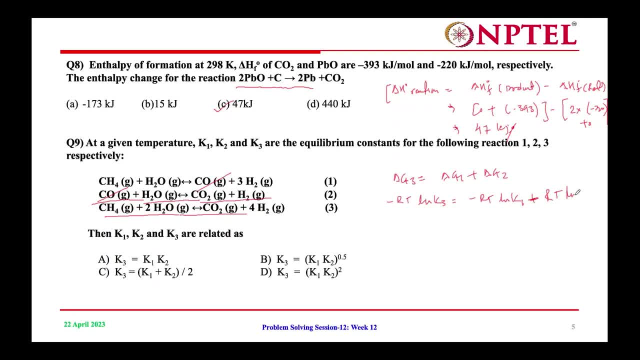 R T ln k 2 right. this gate cancels ln k 3. ln k 1 plus ln k 2. ln k 3, equal to ln k 1, into k 2. k 3 is equal to ln k 2 plus ln k 3, equal to ln k 1, into k 2. 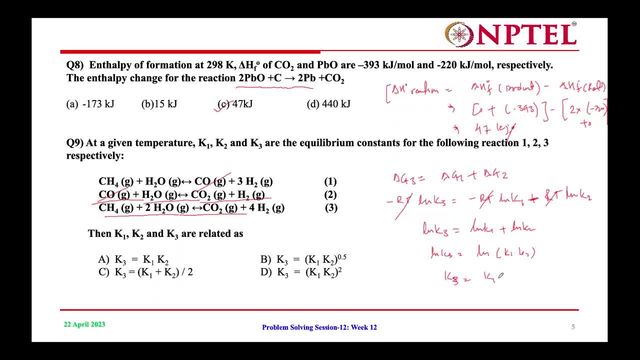 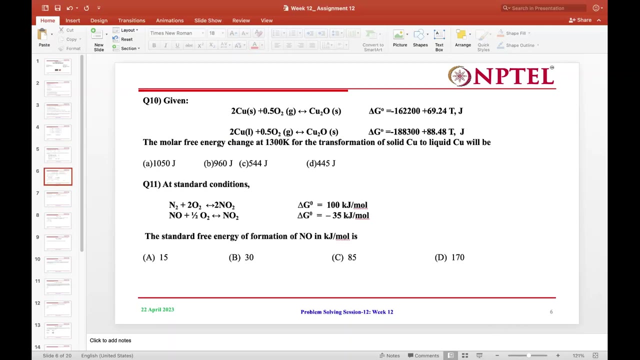 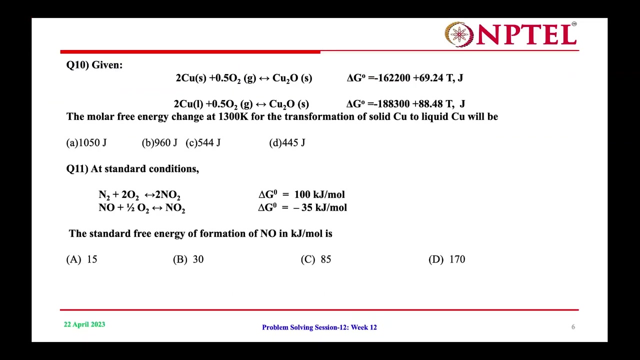 k 3 is equal to ln k 1 plus ln k 2. take the options. so here is the correct answer. I will have to cut clear, sir. okay, good you. Question 10, the chemical reaction given by Cu plus 0.502 gives Cu4 and it is a reversible. 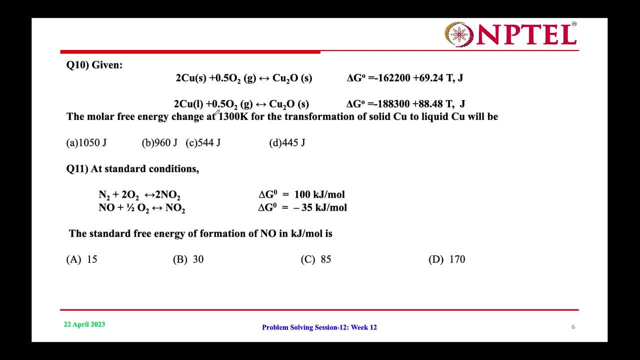 reaction, The molar free energy change at 1300 kelvin for the transformation of solid Cu2 to less Cu will be. so you have to calculate delta G right here. So here really, given the relation for the delta G and reaction, 1 and 2 is like equation. 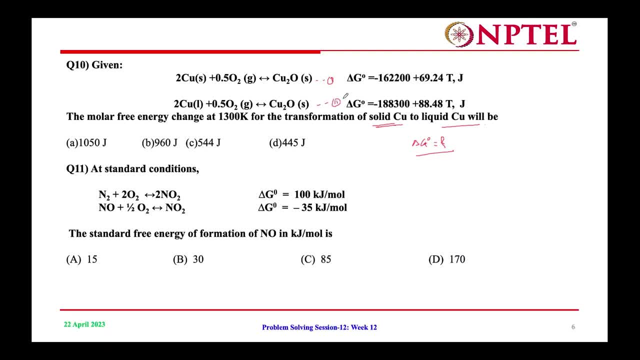 1 and equation 2, or reaction number 1 and reaction 2.. Now here is the transformation: solid Cu to liquid Cu. it means that we have to minus 2.. Sorry, it means we have to proceed. equation 1 minus equation 2. right, so liquid cancels. 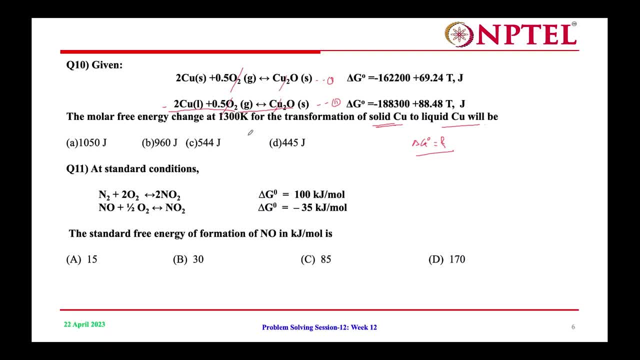 the two cancels. so this is Cu yes twice. So for this reaction we have to calculate the molar free energy change at 1300 kelvin. So similarly, equation 1, equation 2, this is the reaction 1 and reaction 2.. 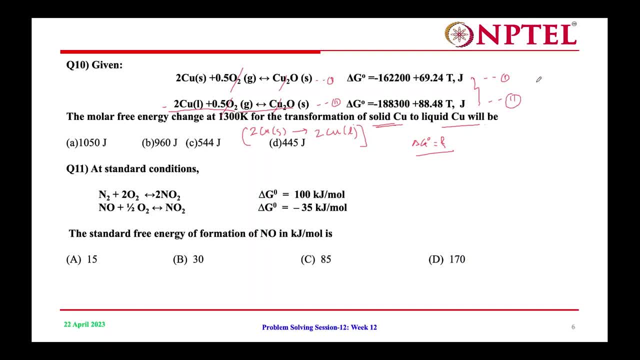 So this is the reaction 1 and reaction 2.. So this is the reaction 1 and reaction 2.. So this is the reaction 1 and reaction 2.. Now 1 minus 2.. We have to Sometimes equation 1 minus equation 2, then you will get a equations delta G. 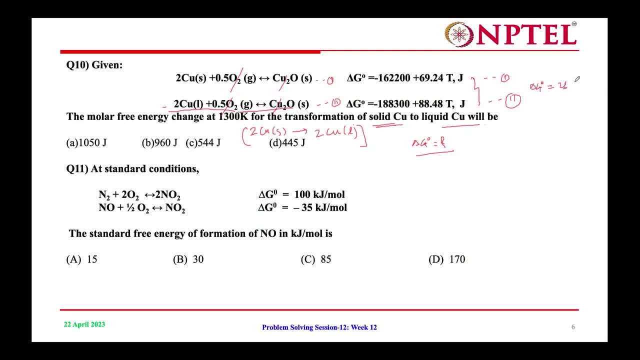 1, 6 minus 19, point 2, 4 C right. Put the value of, So put the value of this 1300 in this equation, below the point delta G, 108 Joules for the two moles. This is for the two moles per delta G. 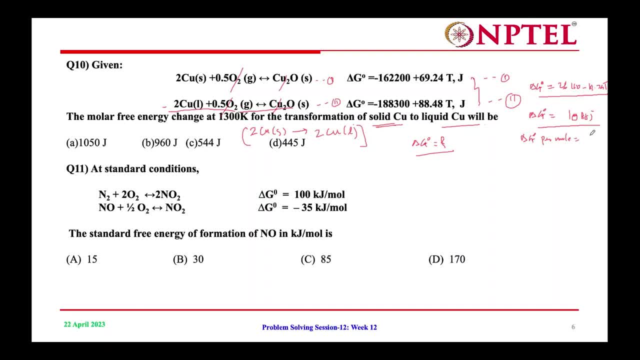 per mole equal to 544 Joules per mole. right Option C item. Now question number 11: at a standard conditions, N2 plus twice O2 gives twice NO2 and delta G given, and NO plus 1 by 2 O2 gives NO2, reversible reaction and delta G given. 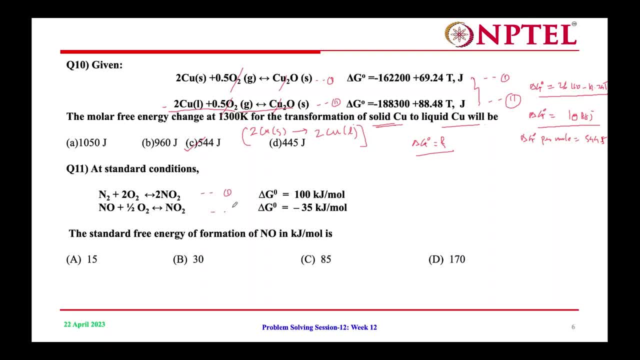 So this is a chemical reaction number one and reaction number two. The standard free energy of formation of NO in kilo joules per mole is equal to delta G for reaction 1 and reaction 2.. So in a given the delta G for reaction 1 and reaction 2.. 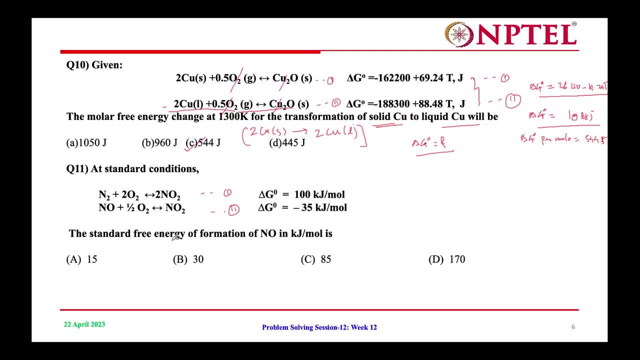 So we have to calculate standard. the free energy for formation, You know so here is a in product, No is a, you know, so I have to make a changes. So in a reaction number once. So multiply by 1 by 2.. 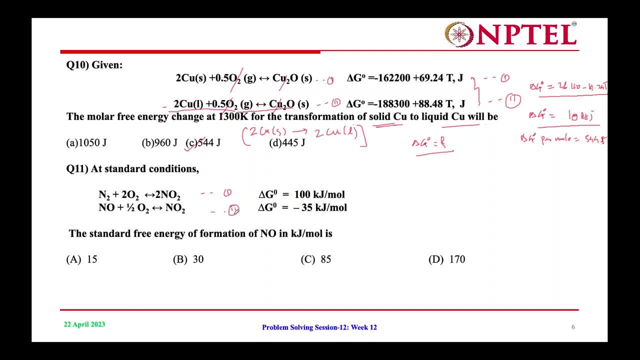 And a impact and reaction to exchange the reactant And product feature. Equation 1 multiply 1 by 2.. 1 by 2.. N2 plus O2.. NO2 right And the reaction And the reaction to exchange. 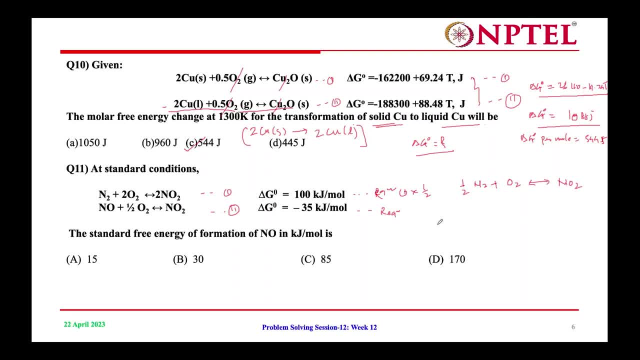 A, reactant, N, Product, each other's N2.. NO, 1 by 2, O2.. Formation of NO right. Similarly for this delta G, there 1 by 2.. And it exchange means it get a positive right. 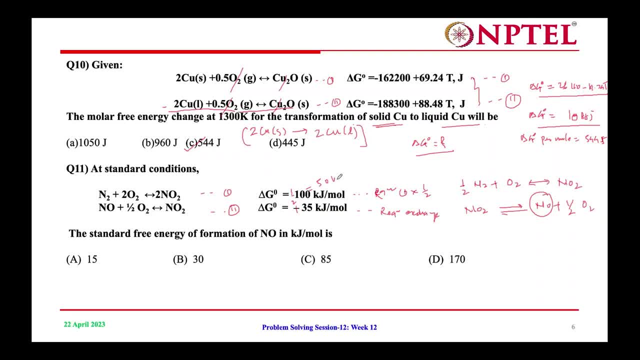 It's a 50. Kilo joule per mole. Now Add a reaction, Just Reaction number 3.. 3 and 4.. Now add reaction 3 and 4.. We need to integrate cancels By 2 N2.. 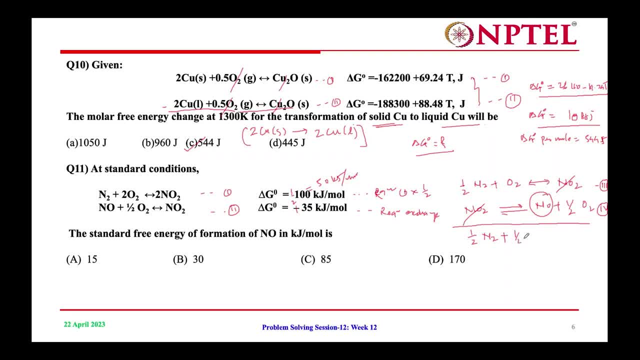 Plus Half O2.. Right, You know Right. So add Delta G When a reaction 1 and 2.. When a reaction 2 and 3. Well, If all the reaction 3 and 4.. Uh, Delta G. 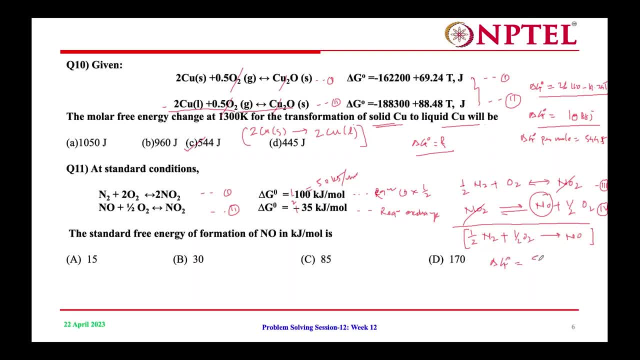 Equal to 50 plus 35.. 85 eurojoules, Or No? Uh U, Uh, Uh, Ah, Yeah, Yeah, Yeh. And so Just say: How about that? Yeah, Yeah. 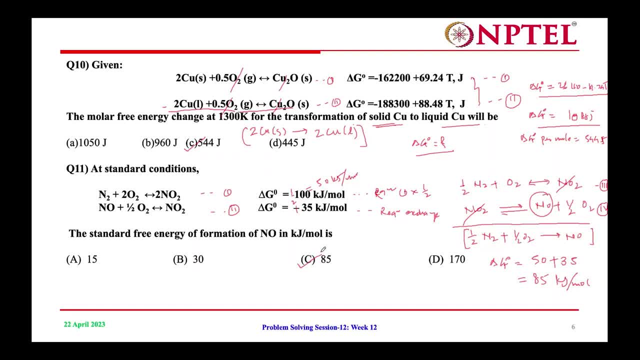 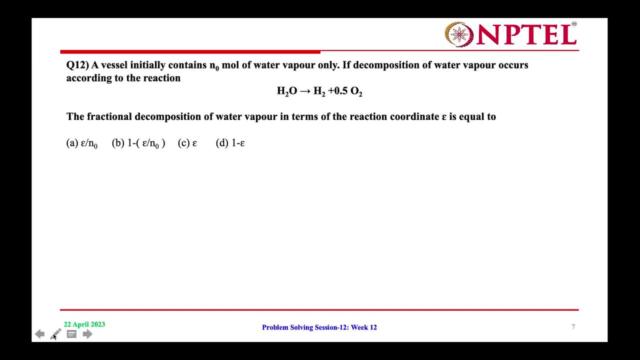 Yeah, All have you got clear? Yeah, Yeah, Yeah, yeah, Yeah, No, No, No, No, No, Yes, No, No, No, No, No, No, Not. Now question number 12,. a vessel initially contains, did not, moles of water vapor only. 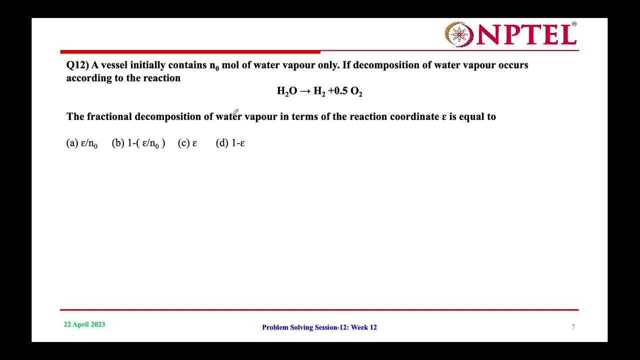 if decomposition of water vapors occur according to the reaction H2O, use H2 plus 0.502.. The fractional decomposition of water vapor in terms of reaction coordinates is equal to. we have to derive the expressions right, As you know. mole fraction is equal to n? i total moles equal to n? i of species initial. 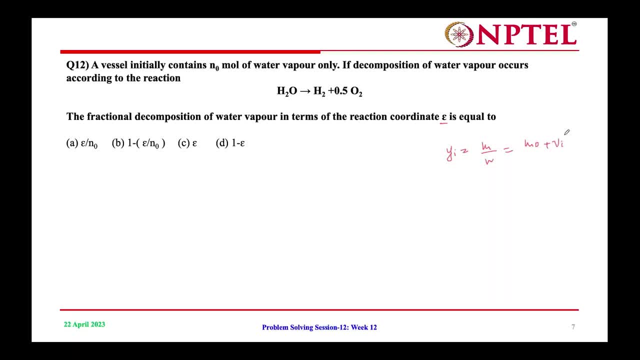 mole fraction plus stoichiometric coefficient into reaction coordinate, plus initially total moles plus total stoichiometric coefficients into external reaction Right- So total moles and initials are not given right- And stoichiometric coefficient for the reactions minus 1 for H2O, plus 1 for H2N. 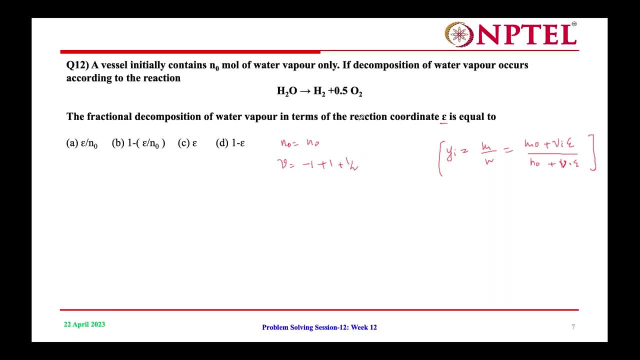 Right, So 1 for H2N plus 1 by 2 are O2, you know, 1 by 2, right. so here, as for the fractional decomposition of water, how to calculate? so NO water initially minus here, CH2 moles of water and initially water presence. 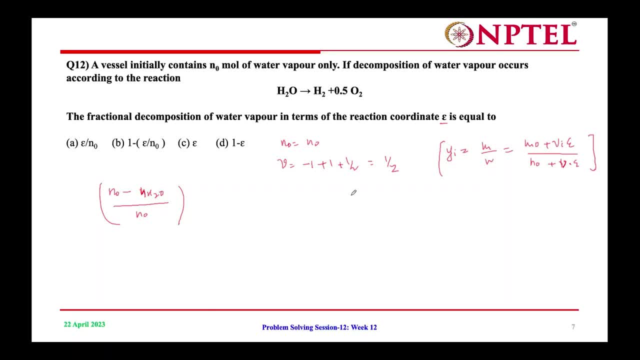 now I have to calculate for water moles of water after reacting. so initially, presence is NOT so in a reactor. so that's negatives and active stoichiometric coefficient is 1. how could this equation, that's a N-NOT reaction equal to 5 fractional decomposition of water vapors. 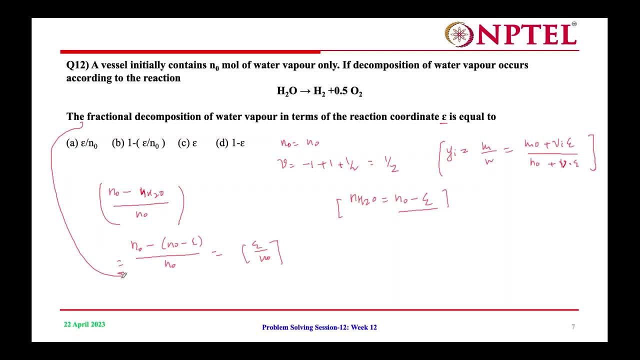 right, so the泉 will come out of here and the N-NOT will come out from this. so this is the total temperature of the water. this will be equals to N-NOT. so this is the final temperature we need to calculate for the you want to use this. 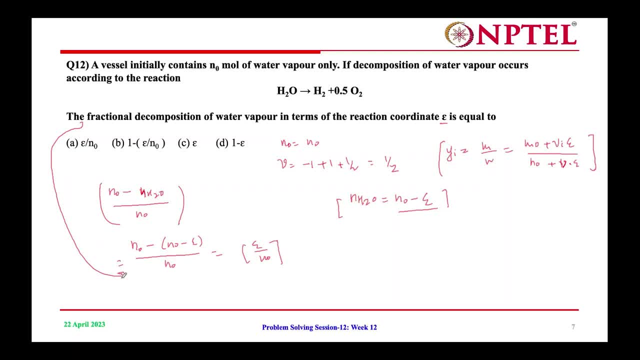 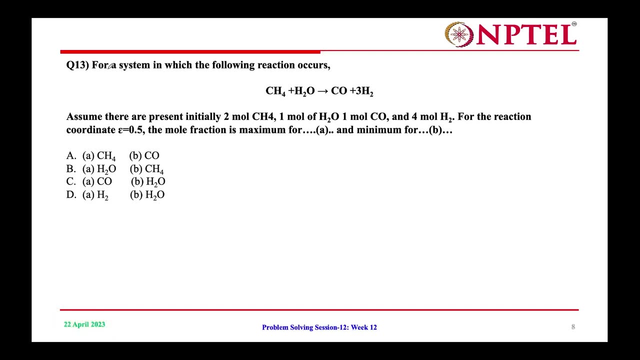 so you want to use this to calculate the temperature for the. you want to use this. we have here. you want to use this to calculate N-NOT. Question No.13 For the systems in which of the following reactions occur: CH4 plus H2O gives CH3H2O, Assume there are present initially two moles. 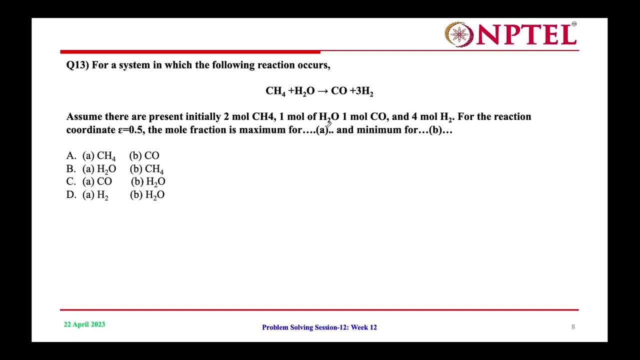 of CH4, one mole of H2O and one mole of COO and four mole of H2O. for the reaction coordinate equal to 0.5, The mole fraction is maximum for and minimum for A. So initially, initially, total small presence is not equal to 2 plus 1 plus 1 plus 4 equal. 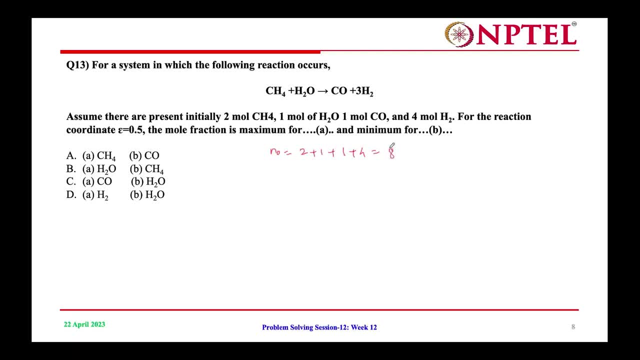 to 8. Total stoichiometric coefficient: 1 plus 1 minus 1 minus 1 plus 1 minus 3 equal to 3 plus 3 for minus 2. Now to derive, the mole fraction for each species y is equal to 0.5. 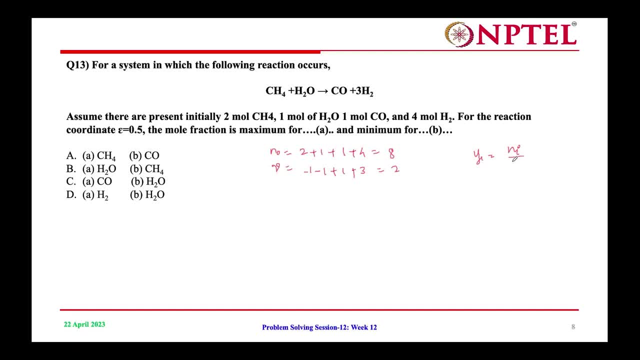 Now to derive the mole fraction for each species y is equal to equal to 3 plus 2 plus 2 X and N, ch2 plus stoichiometric coefficient into reaction coordinate. so Y4, 4. So initially Cs4 is a two moles right psychometric coefficients, minus one, that means minus one. 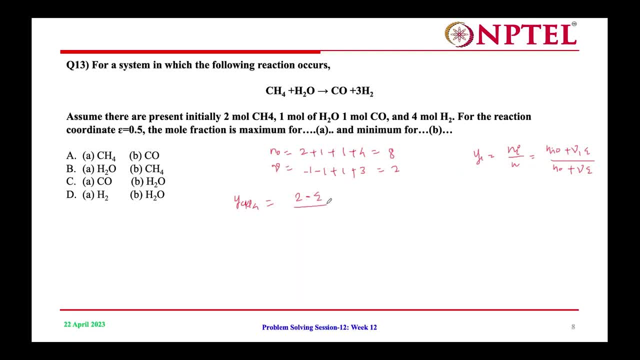 and reaction coordinate. Then initially total moles, initially moles is eight, moles eight and psychometric coefficient two. it's a positive. similarly for the Cs2O: one minus eight plus twice. So Cs2O is a positive and Cs2O is a negative. 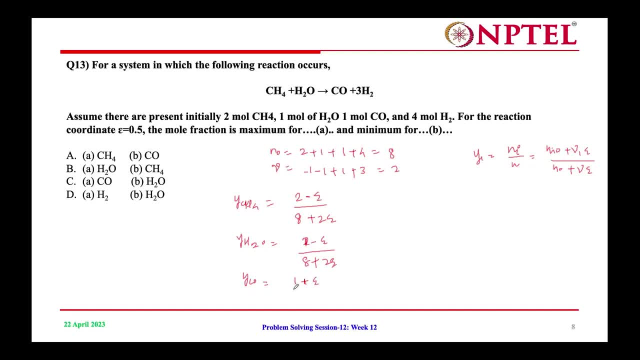 So Cs2O is a positive and Cs2O is a negative. friction by Cs2O initially öğ从 four lower size. here is our psychometric coefficient: p and nitrogen projects, product logit and orangters. So here reaction coordinate value given pi, put null equations. 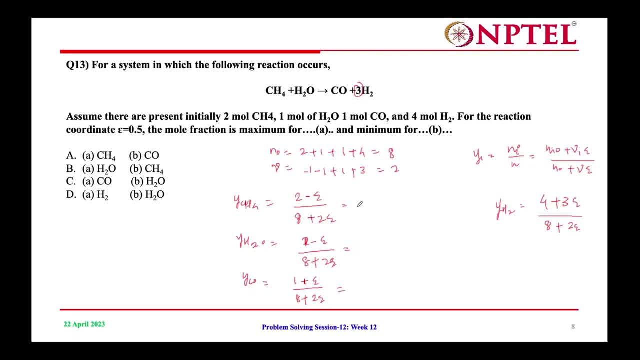 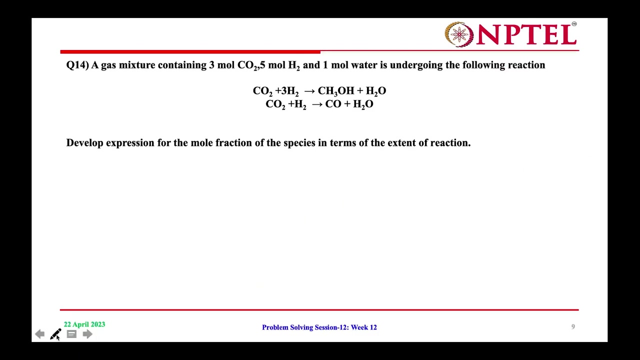 0.16 in H2O- 0.055 and CO 0.16 in H2O- 0.61. the mole fraction is maximum for H2 and minimum for the waters. so option D is the mesh. all of you got clear question number fourteen: a gas mixture containing three moles of CO2. 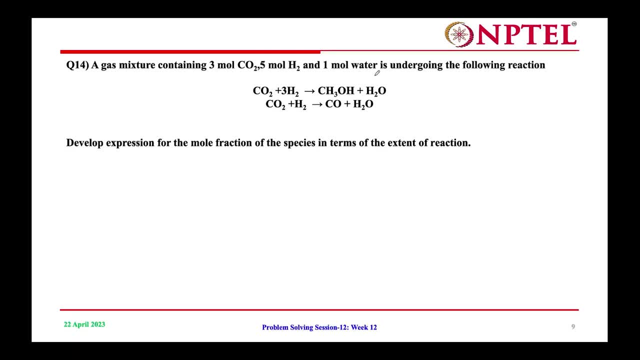 five moles of H2 and one mole water is undergoing the following reaction: CO2 plus H2- use methanol plus waters. and CO2 plus H2- use monoxide and waters develop the expression for the mole fraction as species in terms of the external reactions. 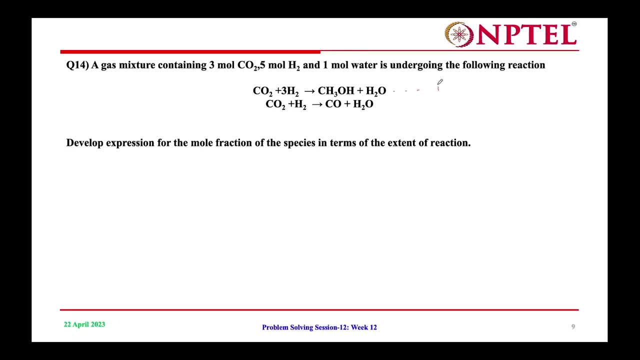 these are multiple reactions, so one reaction, number one, and then reaction number two, eight for multiple reactions. for multiple reactions C and I initially, initially moles of species I plus summation J equal to V. I G reaction coordinate J here uh vij, denote the stoichiometric number of species i in a g reaction right. 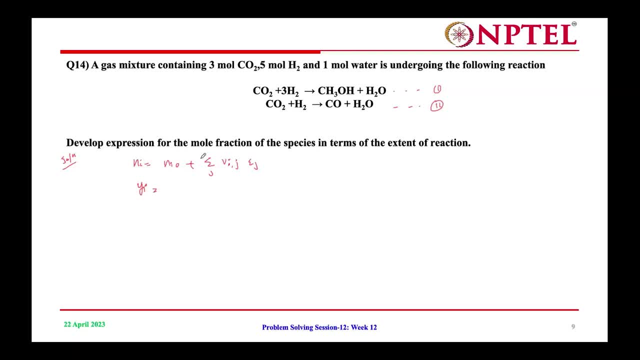 you need to calculate: mole fraction of i is equal to ni of plus summation g, v i, g. initially, mole fraction plus summation g, v i g. reaction coordinate, right now the stoichiometric numbers v, vij. so here i plus co2, ps2, the species. 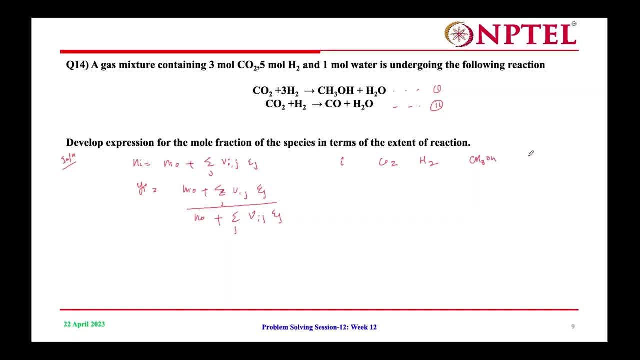 cs3oh, ps2o and co, and j is the reactions, here two reactions. here is the totals. so for so far, this is the tables for the stoichiometric number. well, here co2 is a minus one right and h2 minus three, so you go to one. 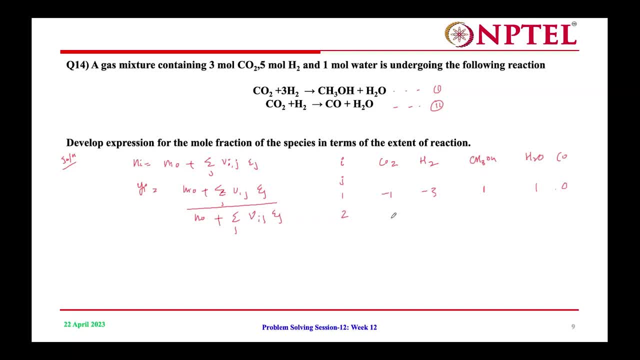 and h2 is one zero, and for second reactions the co2 minus one is two. minus one zero is two, one one. here is the vg totals: the minus two, so minus the one, minus three, minus four, and plus two, so minus two, and my this gets a zero. 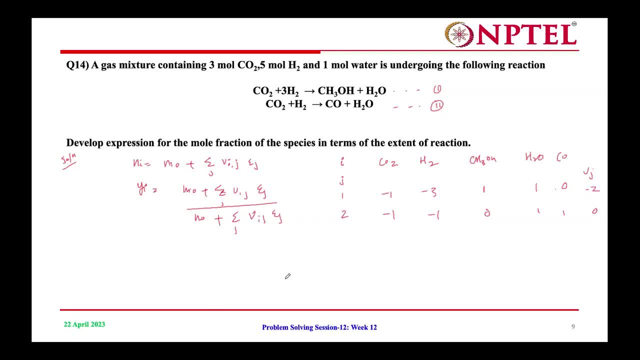 f. okay, at any time you have one again. so those are all satisfy here. and the next one is the possible launcher. now, the total moles initially present after the reacting there will be equal to systems n, 0 plus summation v, g to external reaction. 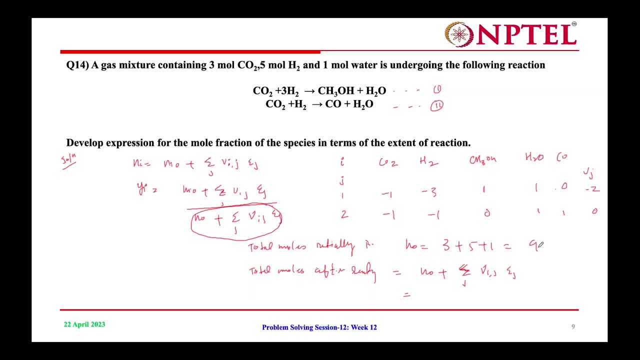 So here is initial was 9.. Right, vita 1, dura 2, panic right and the número cuatro: total coefficient minus two: here is a minus sign, two, one right, because here is a zero right now. calculate for all species for CO2: 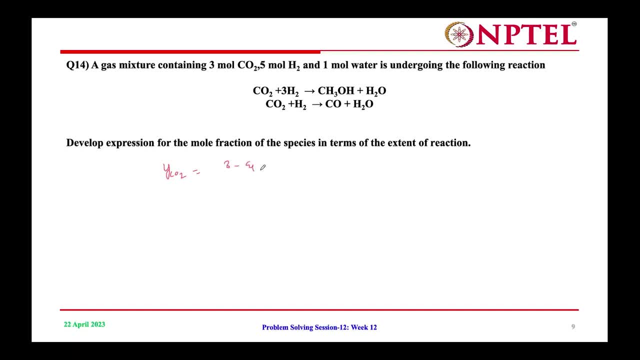 C minus reaction, extent for one is two, nine minus two. y is two. five minus three, two, nine. two. R is two, ohm one plus reaction. extent for one reaction extend for the reaction one plus two, nine. two for CO2, that is for CO extent for reaction two divided by nine. 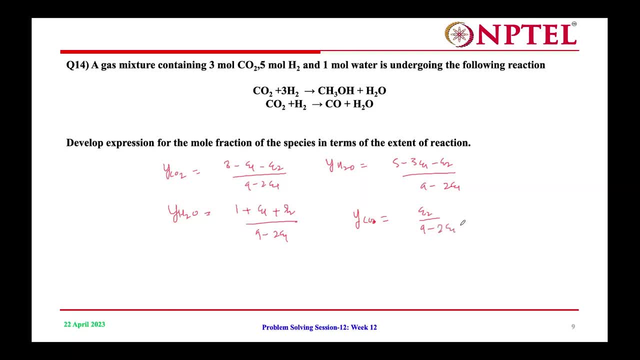 nine minus for C is methanol minus the reaction. so these are the derived expression for mole fraction of species in terms of the strain of the reaction. i'll have got clear. so this is the expression for the multiple reactions. i'm going to the question number. question number 15. 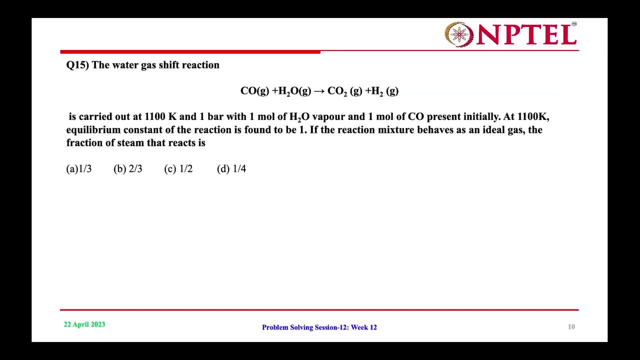 존. the water-gas shift reactions- carbon monoxide plus water gives CO2 and H2B- is carried out at 1100 Kelvin and one bar with one mole of H2O vapors and one mol of CO present initially. the equilibrium constant of the reaction is found to be 1. 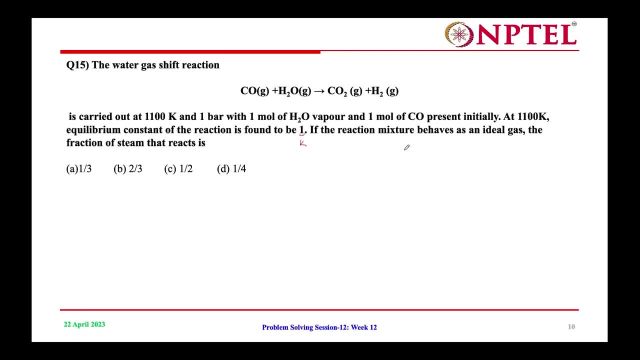 that is ok if the reaction mixture behave as an ideal gas, the fraction of steam that reacts is 1 fraction of this. we have to calculate the fraction of the fraction of the steam that is the reaction. so initially moles 1 plus 1, 2. 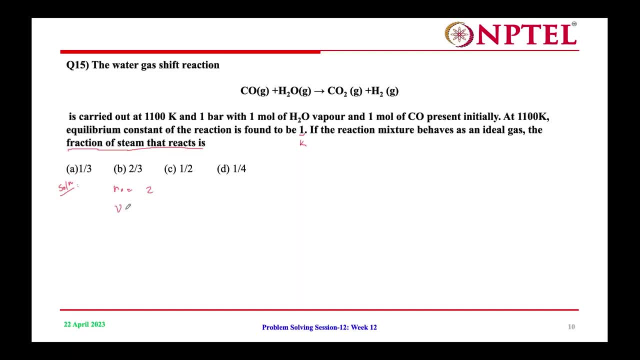 and trichromatic coefficients: age given temperature, given pressure given. so minus 1 minus 1 get 0 minus 1 minus 1 plus 1 equal to 0. now to calculate the reaction, extent of reactions, it is 1. relations k: 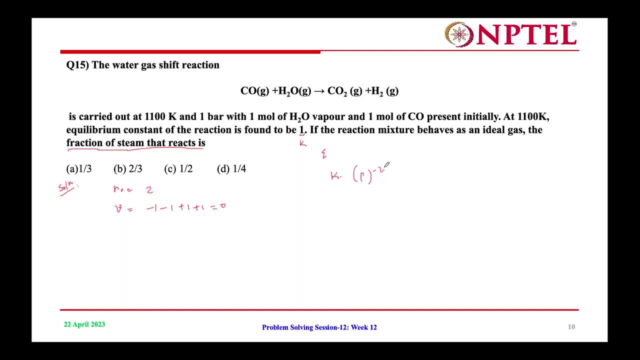 into c: trichromatic coefficients. subscript 2- product submissions. product notations equal to 0. value 1, 2, y, 2, 3, 4, 8, 4, 5, 0, 0, 0, 1, 1, 1, 5, 1. 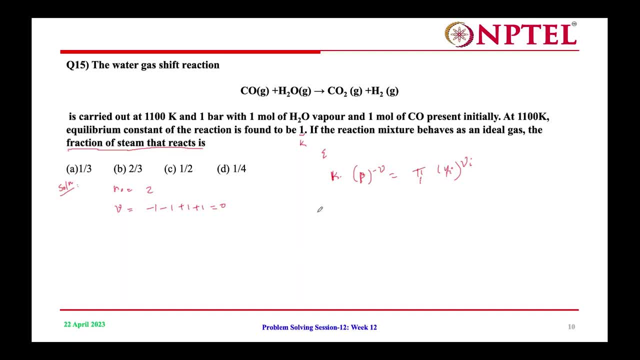 8, 0, 1, 1, 5 expression for the mole fraction of p species. so why gs2o equal to? is there initially one moles and stigmatic coefficient in here? water, water vapor in a reactor, so that's a negative into reaction coordinates into twice and total stigmatic coefficient in zero, so it's a. 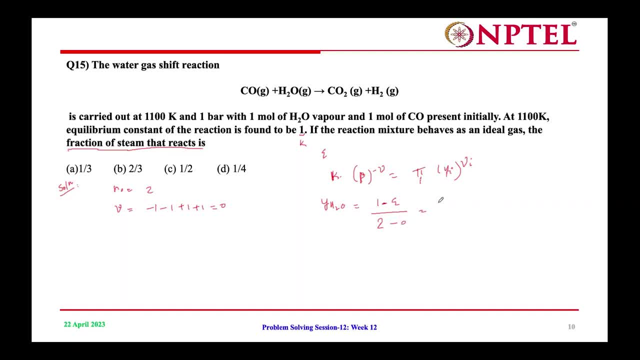 the two, one right, right, vice, yes, same. or y, co2 right. so initial, more initial initials, uh moles up as 0 to h, 0 right reaction coordinate divided by 2, and for y is 2 equal to. now put this equation in this relations: 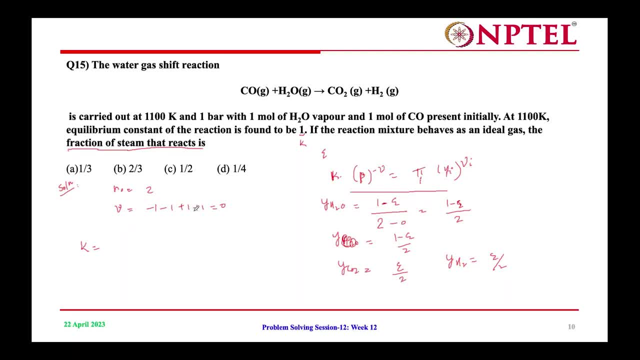 so here, uh. so total stack of coefficient 0, it's the rates of 0. so P is up, it's a 1, 1, 2. why you over 2 into all fashion up? yes to, it's very. is to divide by mole. fraction ups you into mole. 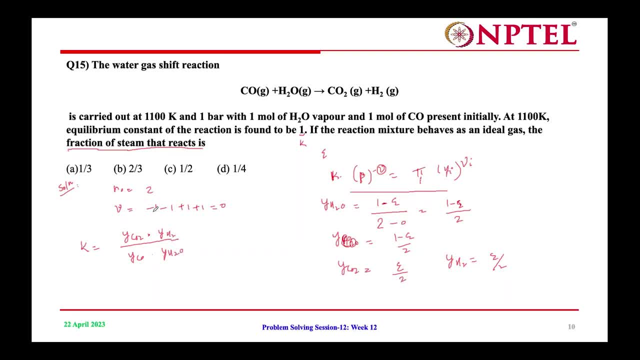 fraction of H2O right pro mole fraction of a product divided by mole fraction of reactor. so put this mole fractions expression in this equations: okay one, and here K is a 1 right. so action of steam that reacts is fine by you. option is the right. 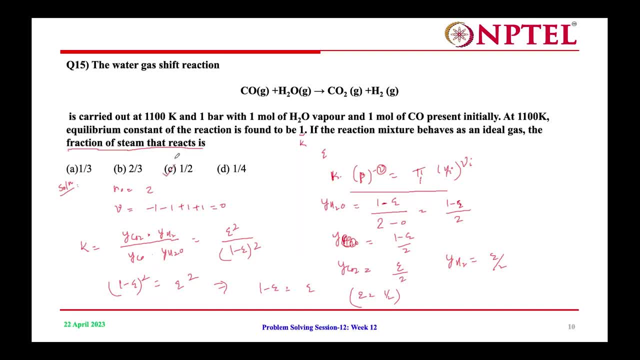 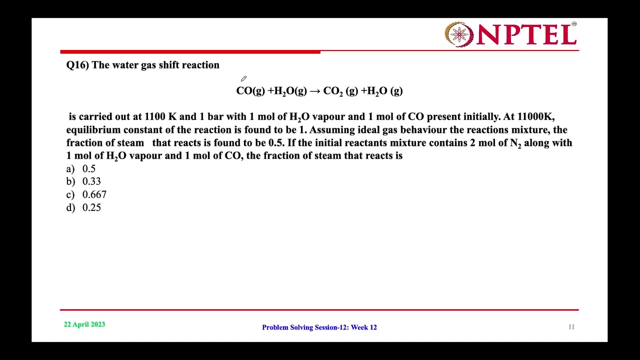 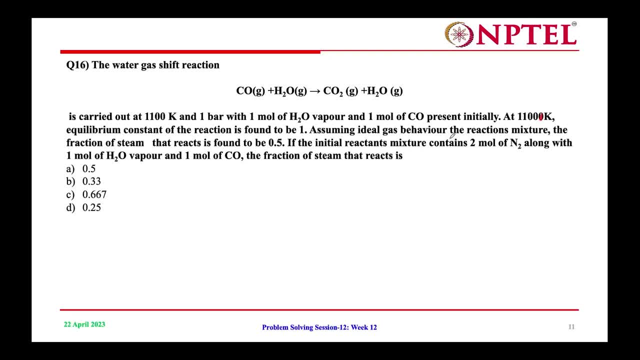 Equilibrium constant of reaction is found to be one Assuming ideal gas behavior. the reaction mixture- The fraction of Steam that reacts- is found to be 0.5.. If the initial reactant mixture contains two mole of into, along with one mole of H2O vapor and one mole of CO, the fraction of steam that reacts. 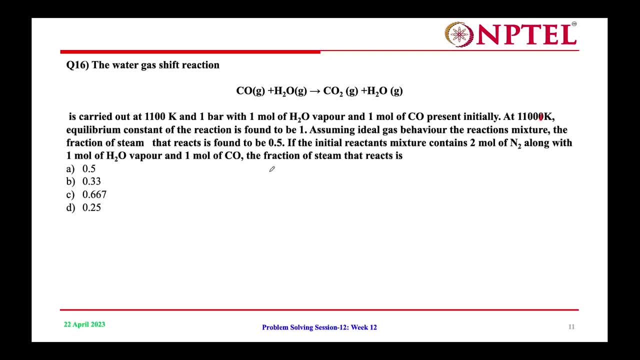 So this statement is same, almost similar to the question number 15.. But here is a extra part: added here Two moles of into, along with one mole of water vapors and one mole of CO. So here N2 does not take part in the reaction and it's a source only as a diluted dilutants. 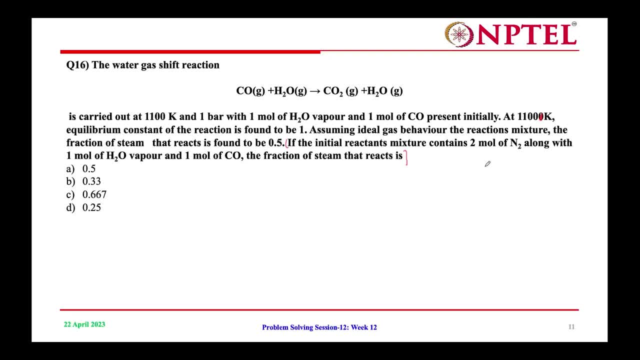 So it does increase the initial number of moles from two to four And mole fraction reduced by the factor two, Right? So here, as far as the faction of steam that reacts it, So it's a Similar to the point five, Right. 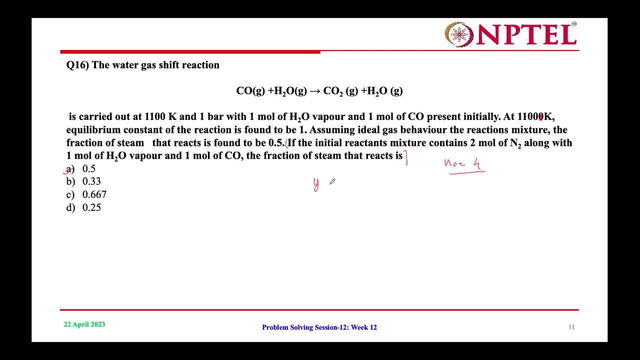 Very power. Why a mole traction up H2.. o equal to one right four. so the four four get cancelled. so you will get relation similar and minus 16 of reaction square, 16 by x square. so i is equal to one. right option is a. 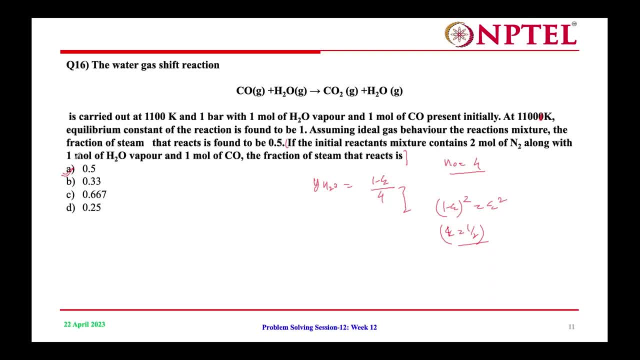 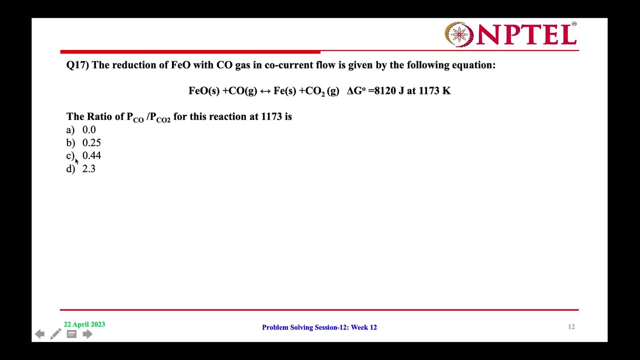 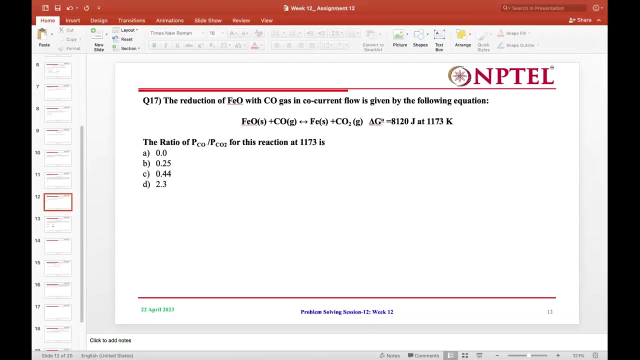 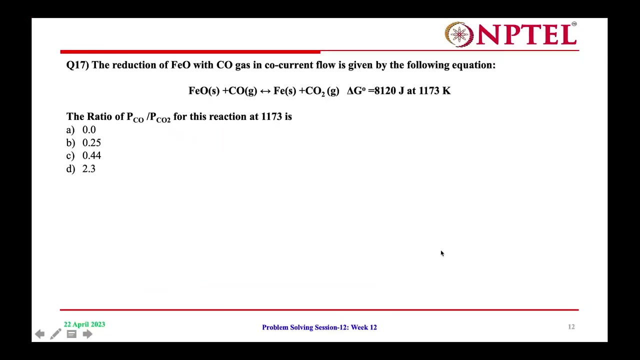 getting or not? you, hey, students, are you there? question number 17.. you, the reduction of a po with co, inner co-current flow is given by the volume indications, the apo plus a, 0 use, ap s plus co2 and synergy. given at this temperatures, the ratio of 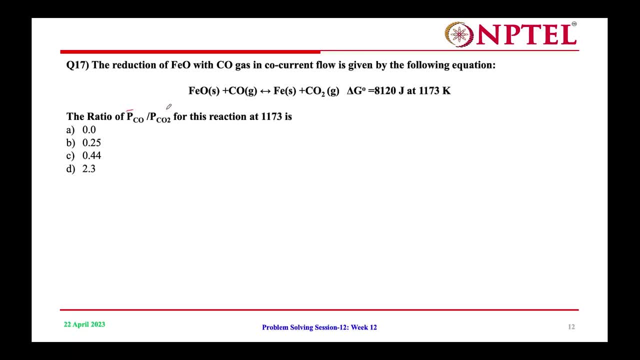 uh po. this is a partial, partial pressure of co and power divided by partial pressure of co2 for this reaction, at this, temperatures option is given. can anybody tell how to solve this one? so in this question, given delta g, given temperature, given right, so we can calculate the. 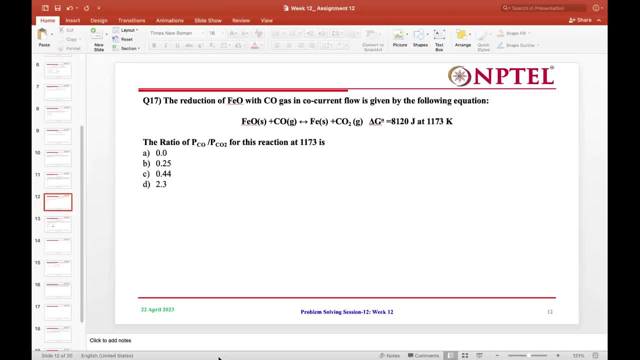 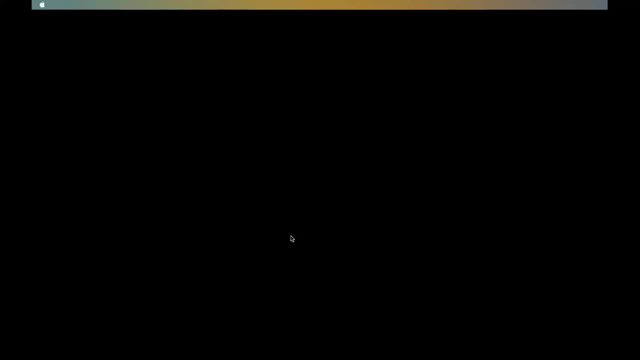 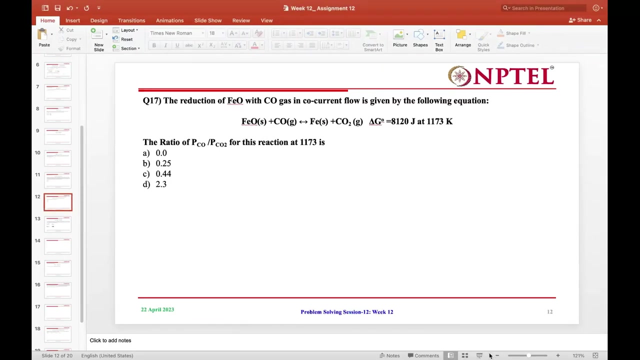 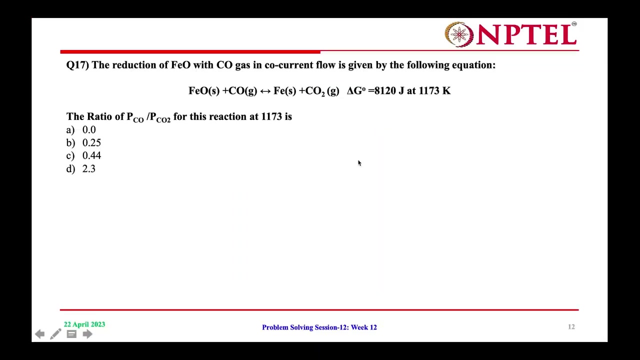 equilibrium constant. you is my slide visible. so in this equation, given delta g and temperatures, so we can calculate uh equilibrium constant using this equation, delta g is equal to minus rt, lf k. delta g given's r is equal to, as constant, 8.31, or is equal to 8.314. 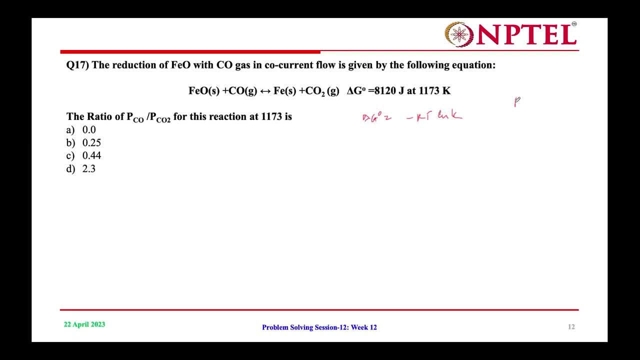 delta g is equal to minus rt, lf, k. delta g given's r is equal to, as constant, 8.31 joules per mole kelvin. so you get k value here. k is equal to 0.435. now, equilibrium constant is related to the fugacity of the components, so k. 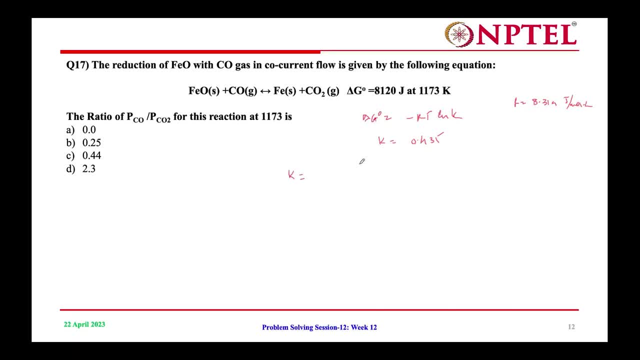 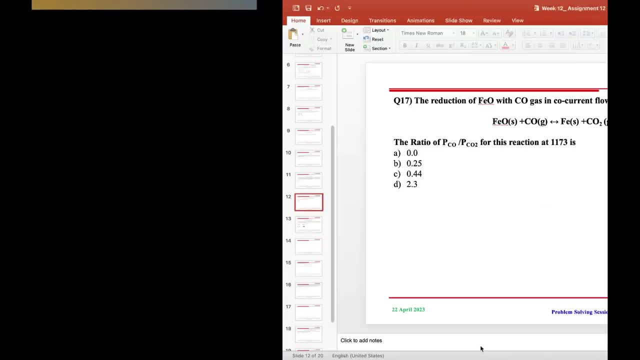 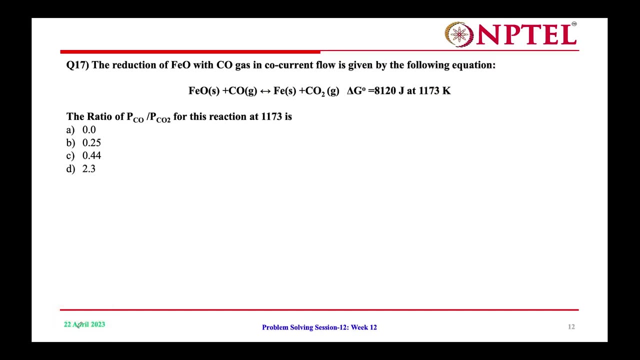 is equal to issue 0.435 k will to product notations to a pi into this relation. so you guys should have solid either one state, y co into pressures, h co into pressures. so mol fraction into total pressure is a partial pressures, so c? co and. 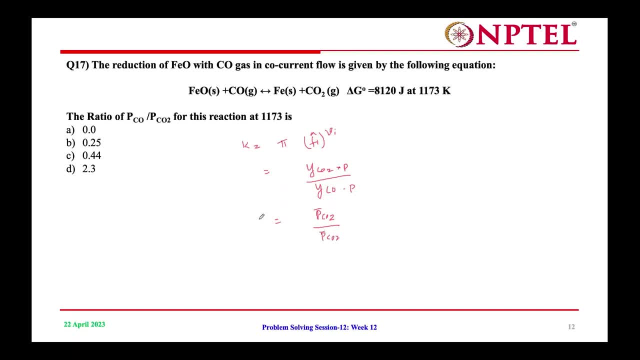 equal to k right and as we calculate the k will do 0.43 in the question at the ratio of pu, co2, partial pressure of co divided by partial pressure of co2, so e co e co2 equal to 5, 0.435, equal to 2.3. 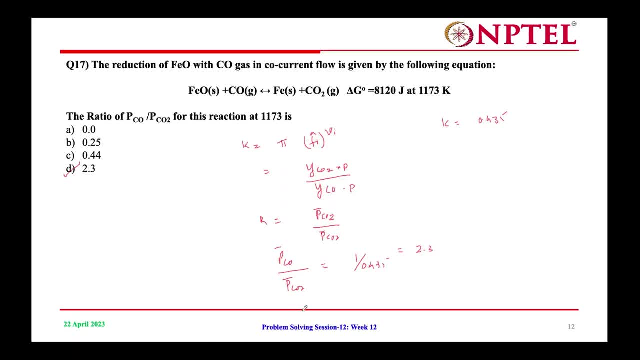 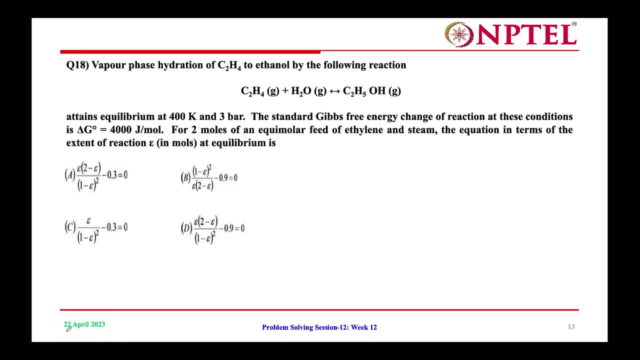 all of you getting this one. question number 18: the vapor phase dehydration of c2h4 to ethanol by the following reaction: c2, ethane plus waters gives a ethanol, but that is the equilibrium. at 400 kilo and three bars the standard Gibbs free energy change of reaction at this condition is delta g equal to 4 and 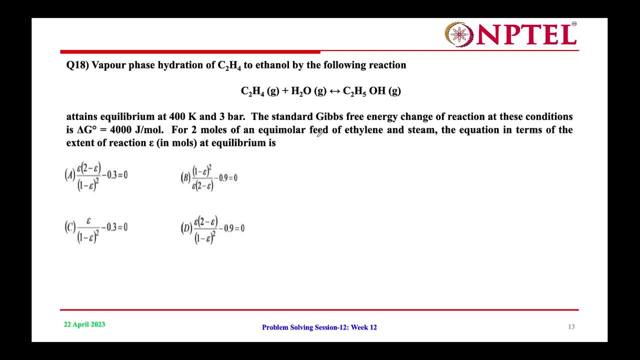 4000 joules per mole are two moles of equilibrium feed up ethylene and steams. here is the equation in terms of the extent of reaction at equilibrium. so we have to derive optional gear right equal to y i. so this is the equation in terms of the extent of reaction at equilibrium, so we have to derive. 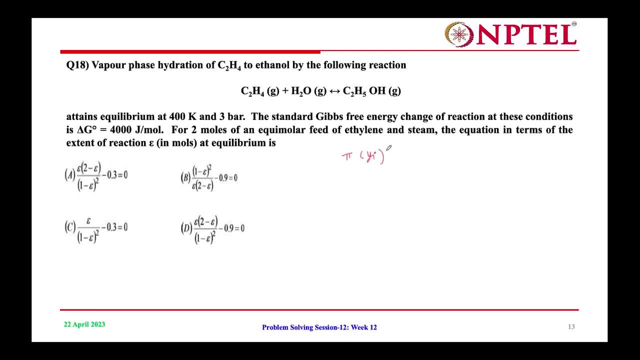 optional gear right into cream. equal to which is blank prime norm less versus prime. yes, that is q. well, and this is q. a should not be boys. i will make it shorter then. 1 barbecue, so this is a, so it's not a significance on these terms. so that's only the thing. 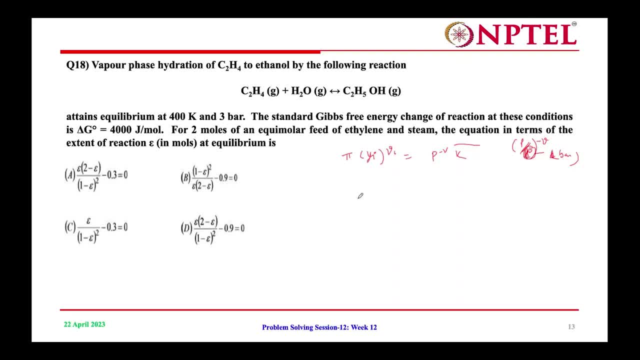 now calculate the first, first equilibrium constant using this equations: delta g equal to minus rt, ln, k. so tip here: temperature given, 400 kelvin, or gas constant, delta g given. so calculate the k value. so k is a point right now for mole fraction, so initially two moles. so 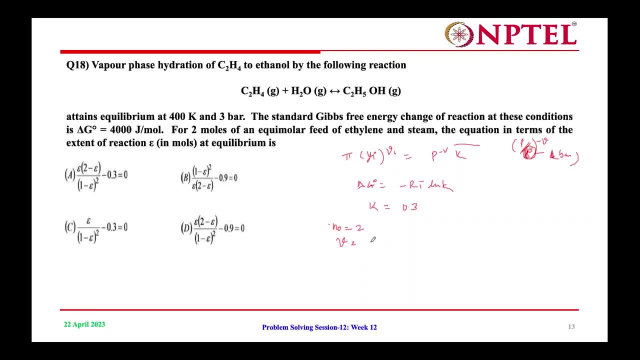 and the stoichiometric coefficient for these reactions is minus one right minus one minus one plus one equal to the minus one. calculate the mole fractions for each species twice t2 h4, so initially one moles of t2 h4 and the reactant z, negative stoichiometric coefficients to action of reaction. 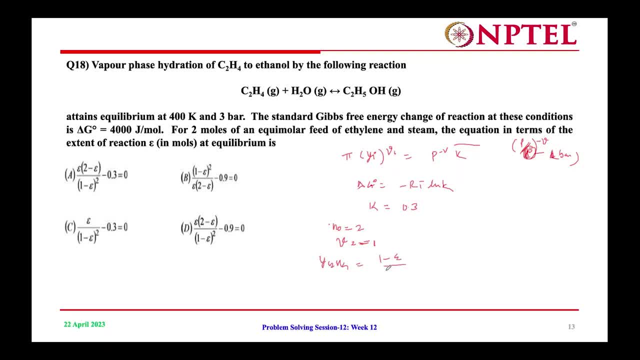 and initially with total moles two and at stoichiometric coefficient a total for this reaction is minus one, minus uh, h2o, equal to same, and for ethanol h5. so initial moles not present here. stoichiometric is a positive for products, the total moles. 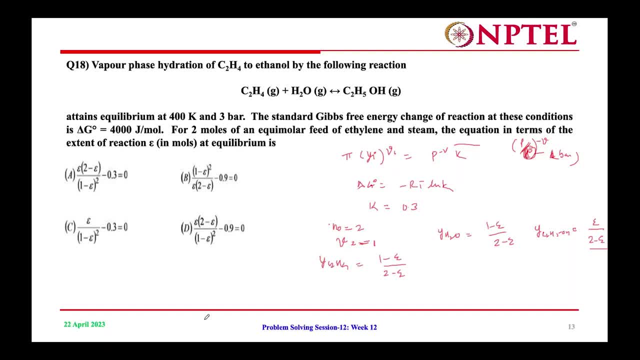 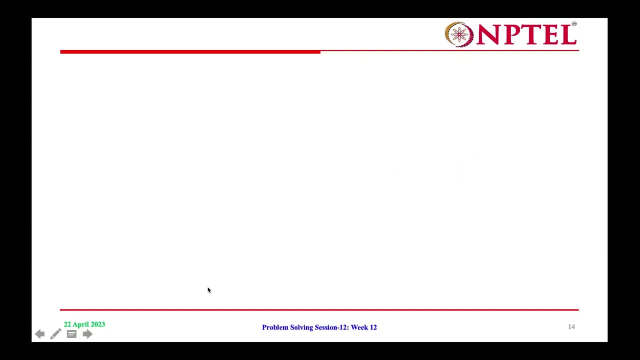 now here is a negative, negative. negative gate cancels and par this is a positive t into k equal to y, g2, h5 moleeste factor of i'm ether. ether降 like little 거 ethanol divided by mole fraction of C2H4 into YH2O. 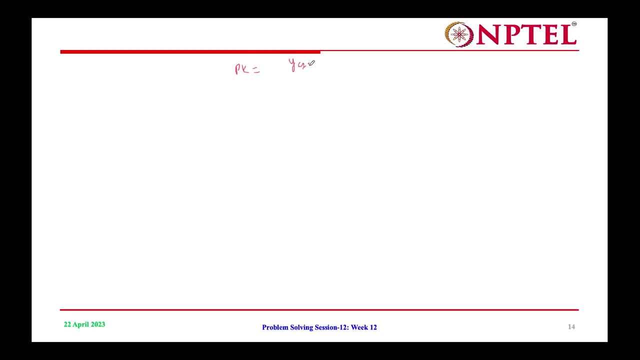 Pk is equal to C2H5OH by C2H4 into mole fraction of the water. so P is a 3 and the equilibrium constant calculated 0.3 is equal to square right 1 minus right. this is a 0.9. 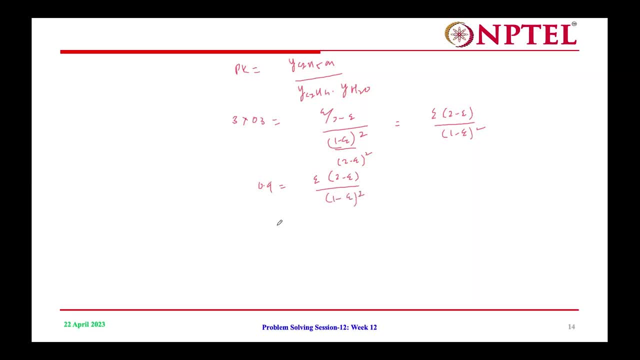 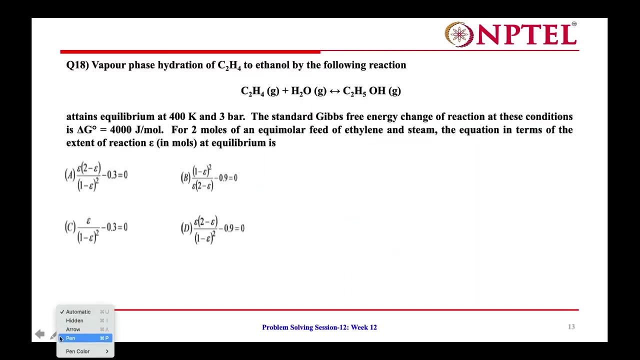 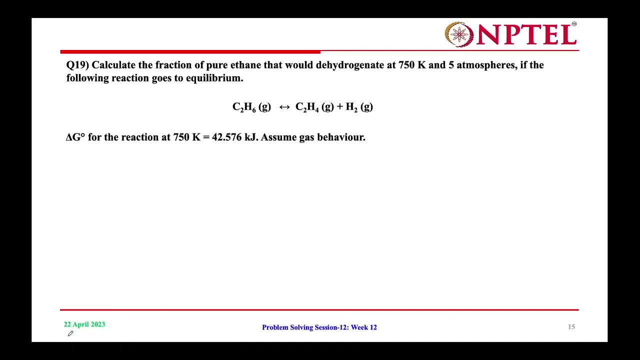 1 minus 2 minus 2.9 equal to 0. we check the options, so these are correct. all of you got clear. now, moving to question no.19: calculate the fraction of pure ethane that would dehydrogenated at 750 Kb. 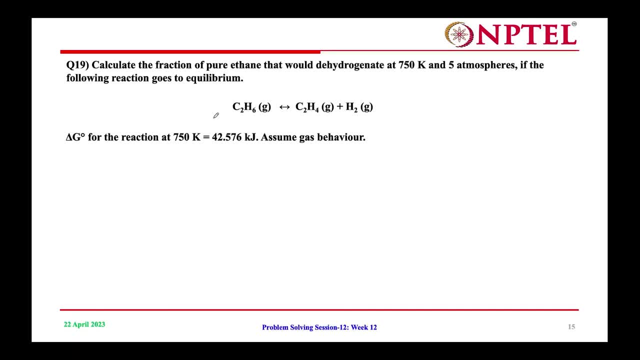 and 5 atm. if the following reaction goes to equilibrium C2H6 gives C2H4 plus ethane as well asrew for delta G. for if the current reaction️ Utah mu, dH2O- change is, Então we show delta g. 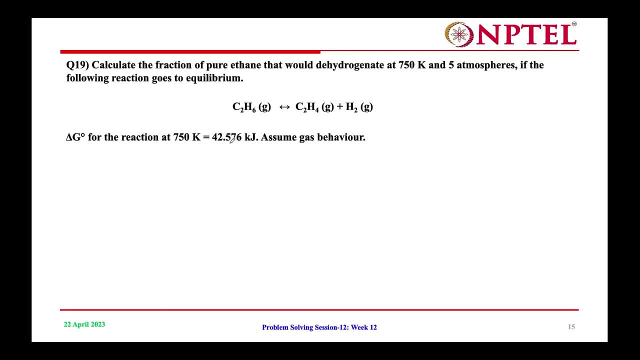 G for reaction at the herex pKm, i means Baldy minus delta, H4 to Atp. MM mechanics didn't get a point here, and delta i am going to too much if we do the procedure here. so for reaction at 750 Kelvin, 42.576 kilojoule, assume the gas. here we have to calculate, calculate. 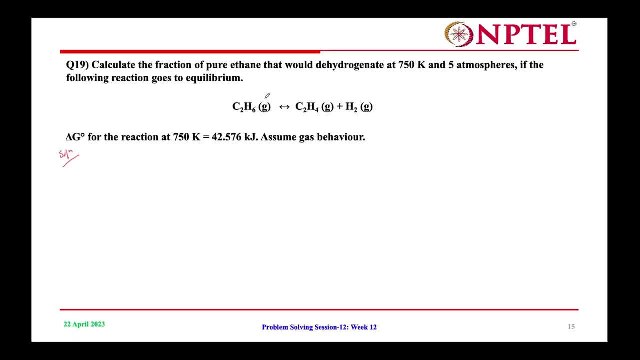 a fraction of pure ethane. so delta G given, temperature given, pressure given, say so, initially, calculate the K value, equilibrium constant, which in the this relation minus RT, Elan, okay, it's equal to zero point nine, nine, eight, two right, and here consider the one, moles of a. 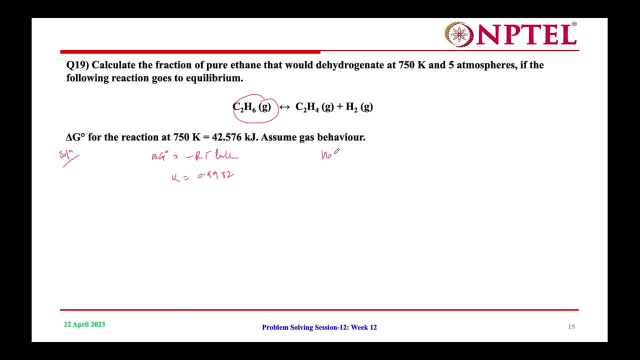 Ethan patient initially. so not. it's equal to one strychomotric coefficient minus one plus minus one plus one power C, two S, four plus one power two minus three. so one one plus one power three. what do you have to calculate the mole fraction for the? 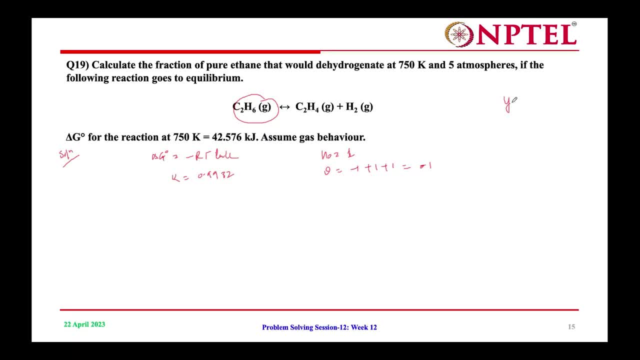 ethene by two, six, right here. so K is equal to the mole fraction of C2H4 into mole fraction of C2H6. right, so here is the v is equal to one, is the minus one. so we can take p- here is same- into p. right now calculate the expression. 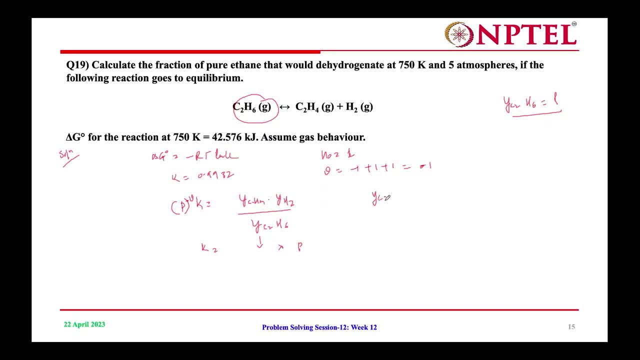 for the mole fraction of each species, C2H6. so initially one moles initially presents one moles, C2H6. the reaction, so psychometric coefficient is minus and here reaction extends and totals moles were one and here is the positive signs, so y is C2H4. 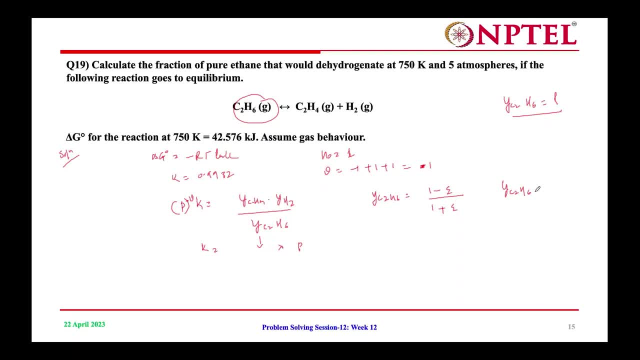 H6, then C4, so initially moles are zero. our C2H4 is zero. so reaction: extend squared by all o plus total mol. reaction: extend squared by 1 plus total mol. reaction: extend squared by 1 plus total mol. now this is the expressions of mole fraction put in the in these equations. so k is a 0.99. 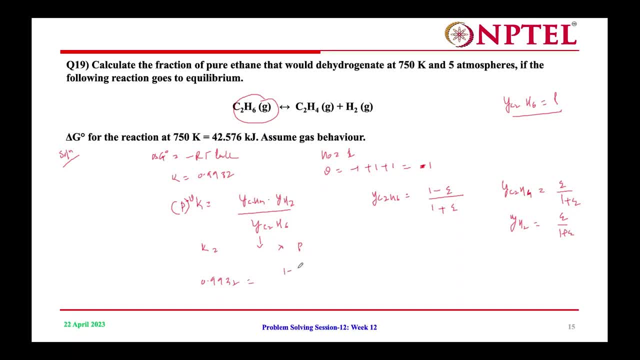 p2 into 1 by 3, right it's the same one. so here, 1 by 5, 1 by reaction extent, right into p is a high atmosphere and all this is the expressions. it phi is equal to pi for 0 and the question: 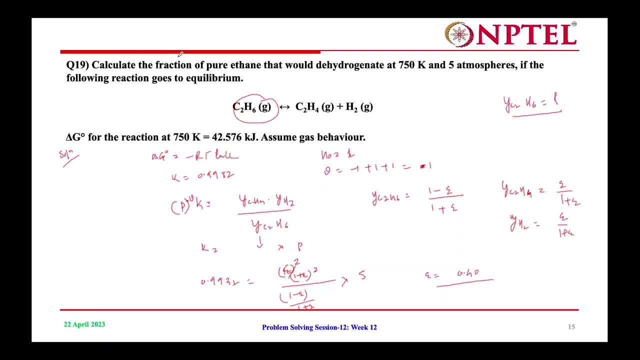 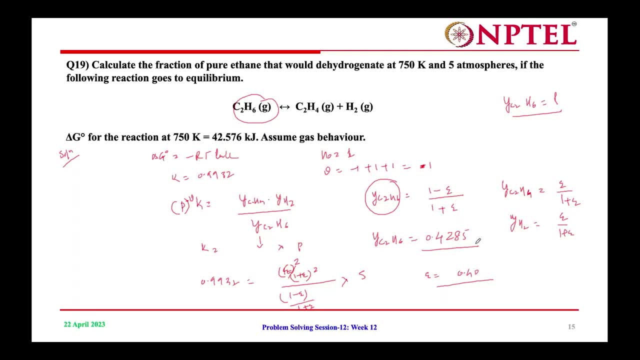 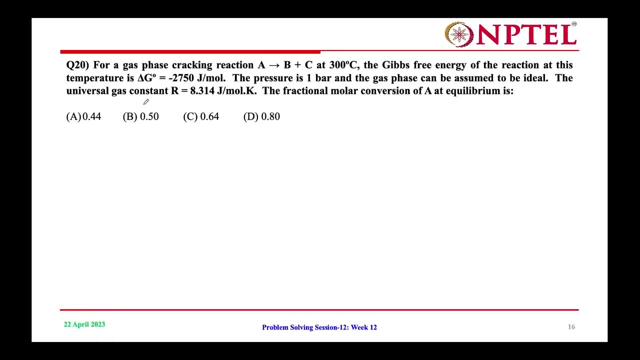 p o p p a a p a p a p p p. moving to the question 20.. For a gas phase, cracking reaction A gives B plus C. at 300 degree Celsius, The Gibbs free energy of the reaction at the temperature is delta. G is: 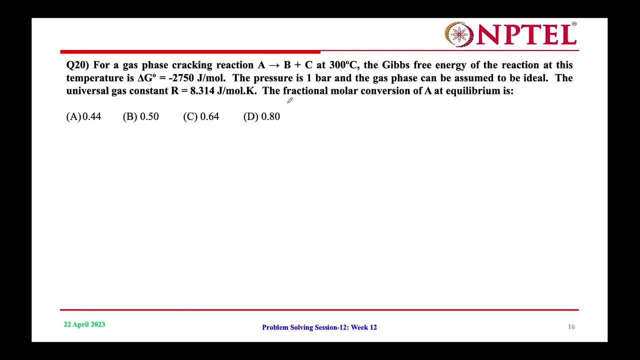 equal to minus 2750 joule per mole. The pressure is 1 bar and gas phase can be assumed to be ideal. The universal gas constant R is equal to 8.314 joule per mole into Kelvin, The fractional molar conversion of A at equilibrium. So we have to calculate the fractional molar. 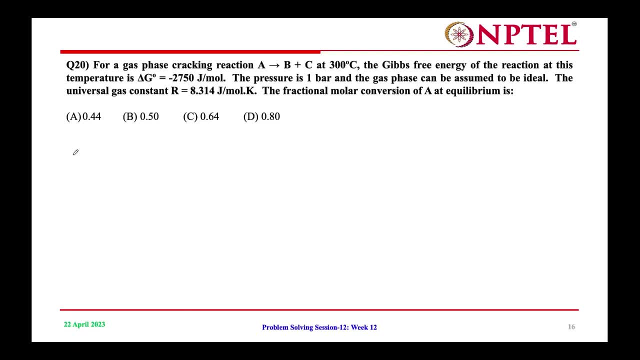 conversion of A at equilibrium. So in this questions we have to use same concept as the previous questions. So first, delta G gamma is equal to minus 2750 joule per mole, The temperature pressure given. So calculate the first bar K equilibrium gas time Equal. 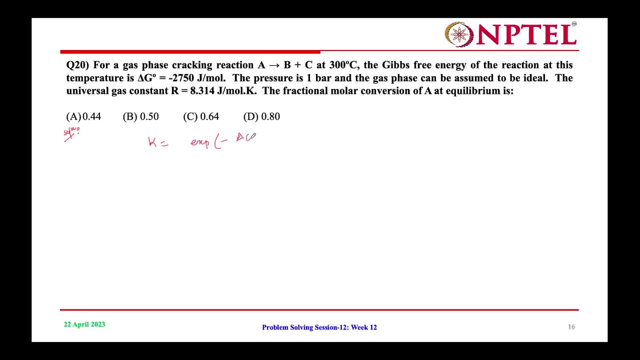 to X Delta C by 30. Put the value We will get: K is equal to 1.7 K. net 1: 0 right Equal. so here total a is equal to one more. it's a pmbc. so a naught equal to one right. 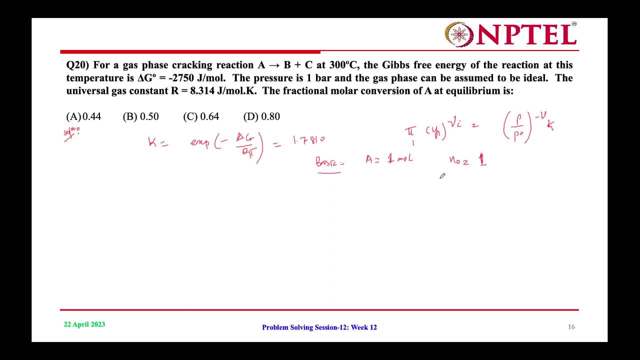 now this p naught equal to one, eight, three, one bar. it's only p. so x is a fractional molar convergence. so this is a species: a, b, c. so like multi coefficient minus one, one, one right the totals initial moles one zero, zero. so p is equal to one. 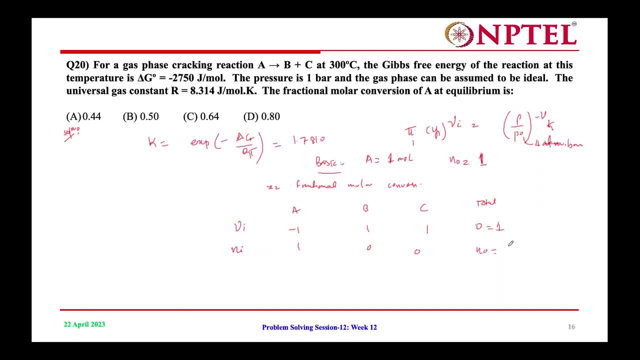 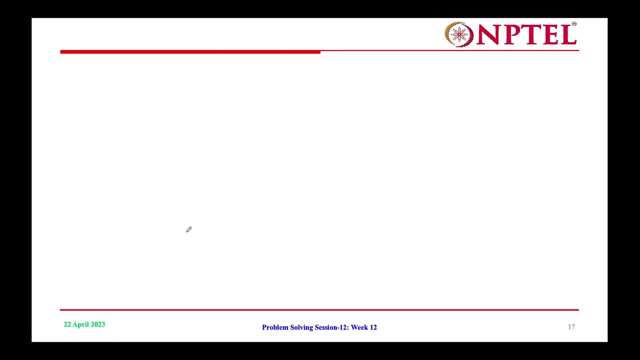 and two, one right, at equilibrium, one minus x, right, x, x and totals: one plus x right and mole fraction: one minus x for total moles: one plus x, one plus x right, right, right, right, right, right, right. now put equations: one point seven, eight, one zero equal to: 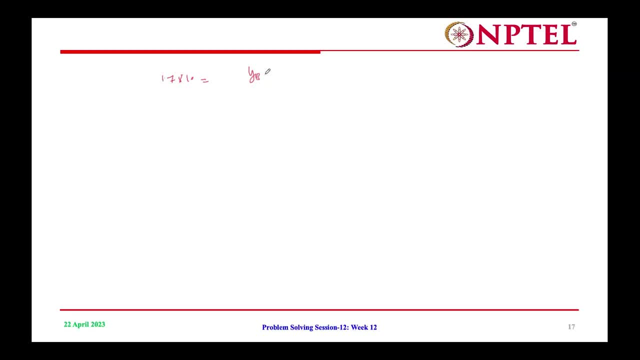 yb into yc by ya x one plus x, x one plus x for my x plus one plus x one and and the. what is the value of the value of the value of p? n and p isn't strong enough right 1 and p doesn't work. calculate that. what is the value of p? 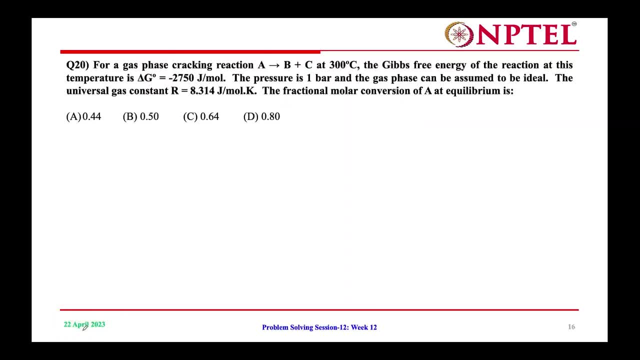 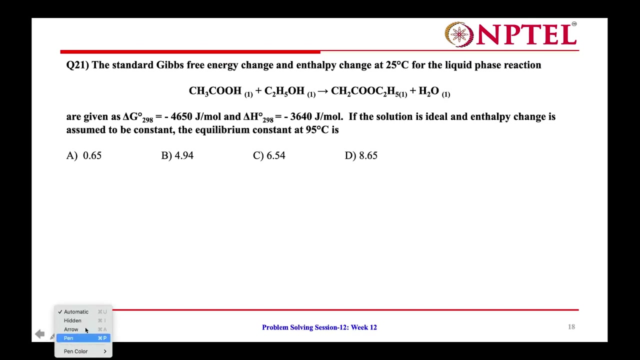 is equal to 0.8, so fractional molar conversion at equilibrium is 0.8. so option D is a right, clear or not? so, going to the last questions, the standard Gibbs: free energy change, the enthalpy change at 25 degree Celsius for the liquid phase reaction. 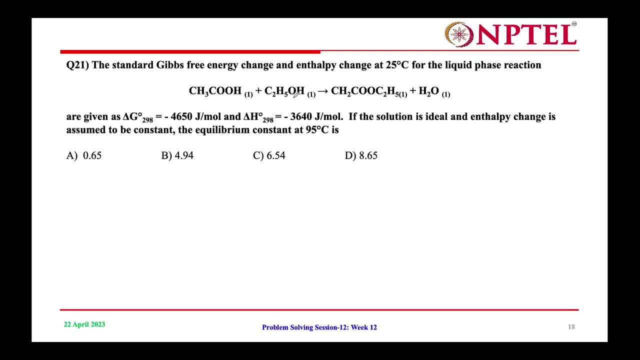 CH3COOH plus C2HOH gives C2COOH5 plus H2O. are given as derivative of C2H5. are given as derivative of C2H5 plus H2O, delta G at 298 minus 465 joule per mole and delta H at 298. 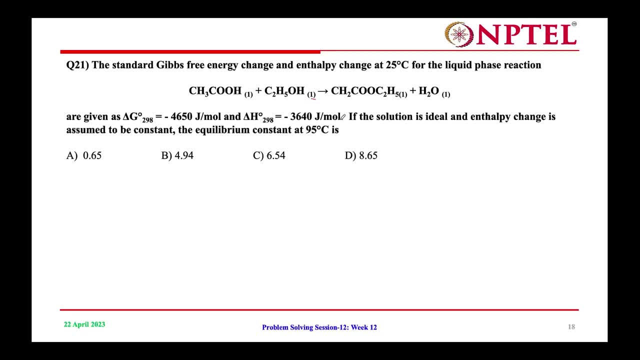 equal to minus 3640 joule per mole if the solution is ideal and enthalpy change is assumed to be the constant, the equilibrium constant, at 95 degree Celsius. so we have to calculate the K value at 95 degree Celsius. so, delta G given, delta H given. 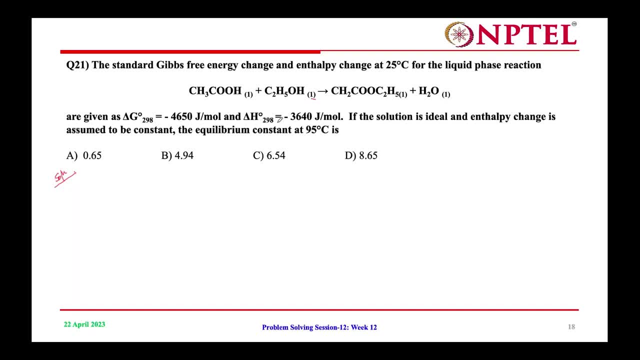 and the standard Gibbs free energy change at enthalpy change at 25 degree Celsius and the standard Gibbs free energy change at enthalpy change at 25 degree Celsius. so there are two relations: K is equal to Xp exponential delta, G, Rt and ln. 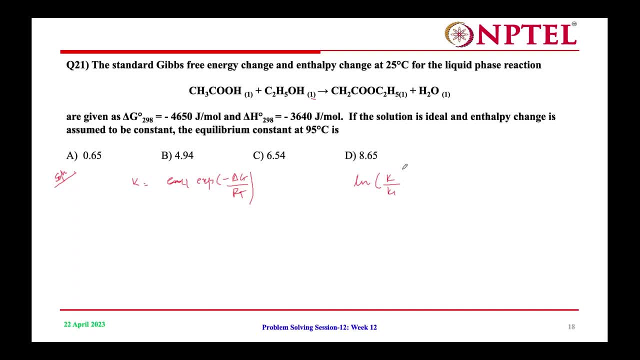 T, T1, delta G, R, 1 by T and 1 by T1, right, so let's calculate the K value at 25 degree Celsius, delta G given R8.314 and T is 25, so convert into Kelvin, so delta K is equal to.